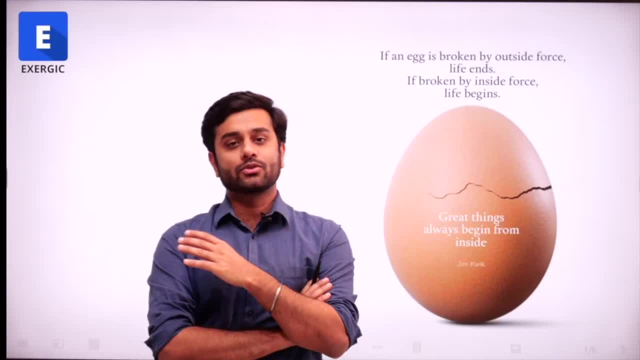 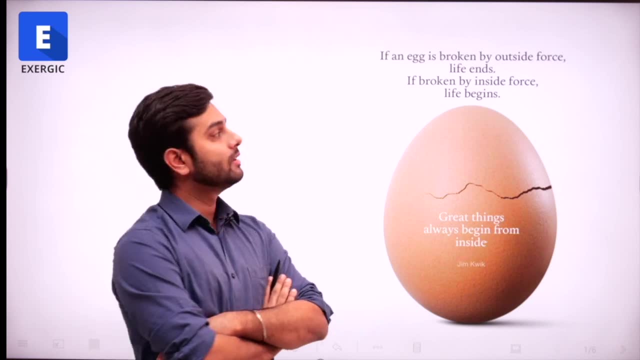 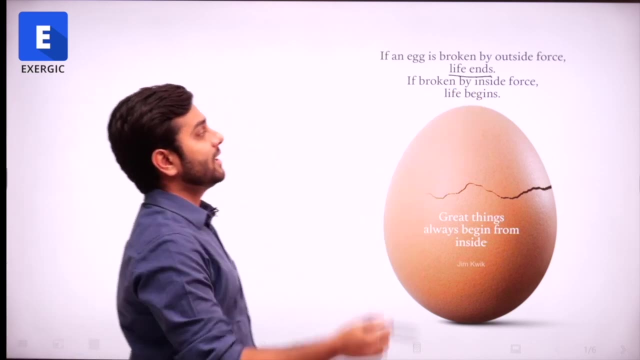 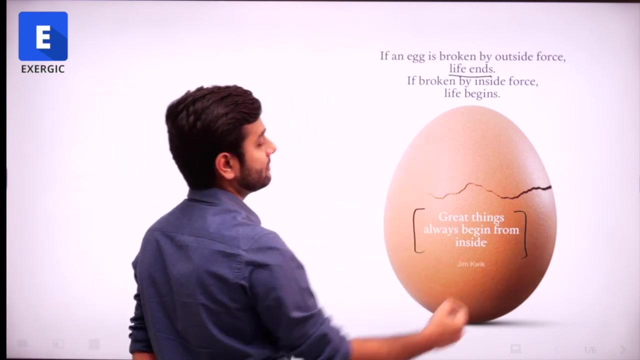 Hello, dear students, Let us start this course by a very beautiful and very meaningful quote, which is written here: If an egg is broken by the outside force, the life ends, But if it is broken by the inside force, the life begins. Great things always begin from inside. What does it mean? 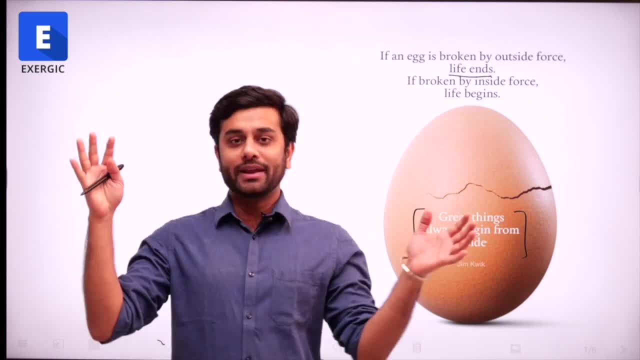 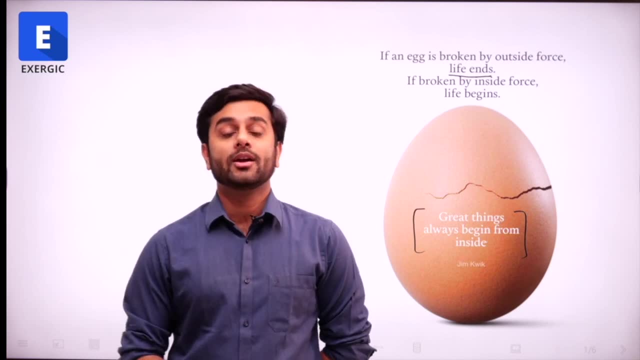 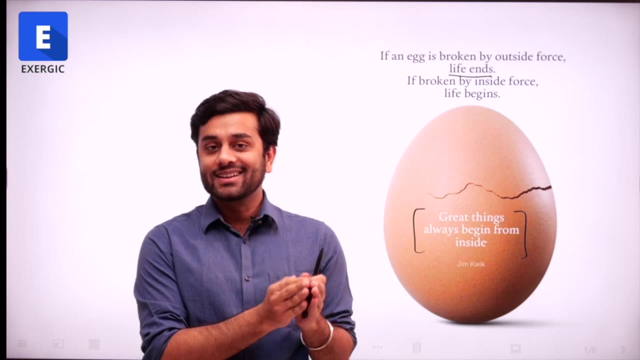 It means that any egg if it breaks from the outside, what happens? The life inside of that egg? it dies, It is the end of a life. But if it is breaking from the inside means whatever living being is within that egg that is opening up the shell That is breaking the egg. It is. 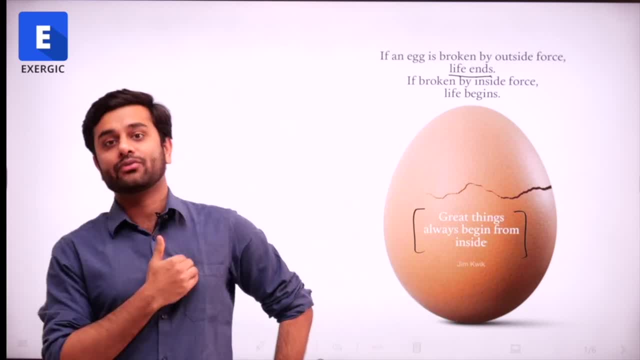 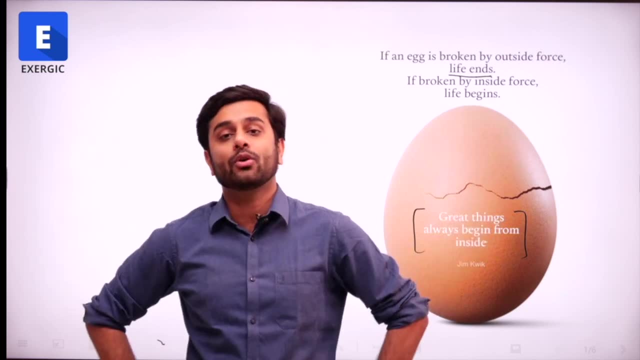 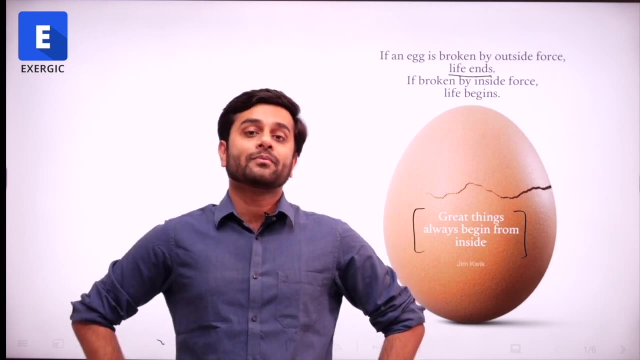 the beginning of a life, So great things always begin from the inside. Always look for inner inspirations and not external motivations. Always look for discipline which comes from within. This is something that you must realize And it is a very important learning for you. 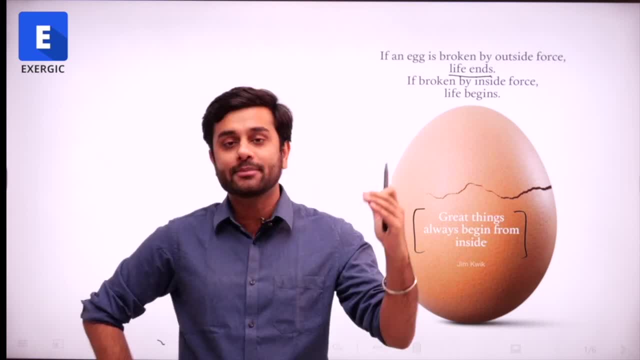 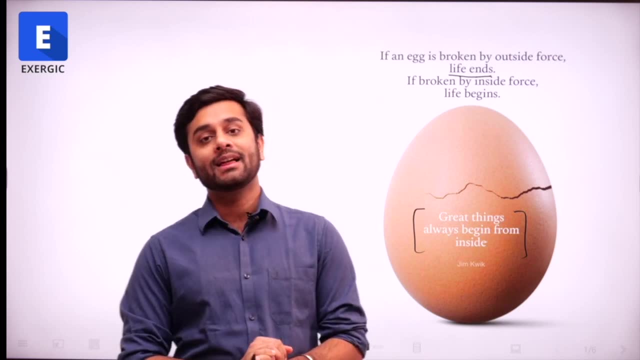 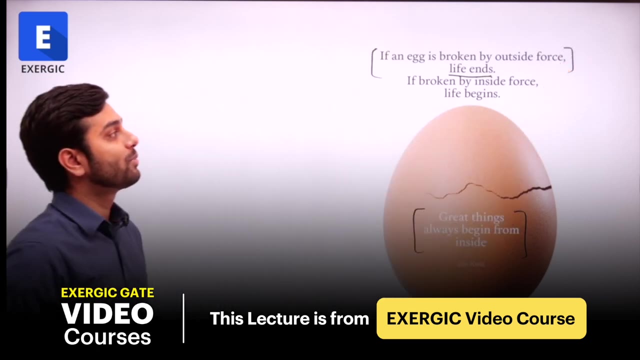 not only as a GATE aspirant or any exams aspirant, but throughout in your life. Now why are we discussing this here in Strength of Materials? Let us focus on the first part, On the first part of this. If an egg is broken by the outside force, the life ends. Any outside force, any outside load. 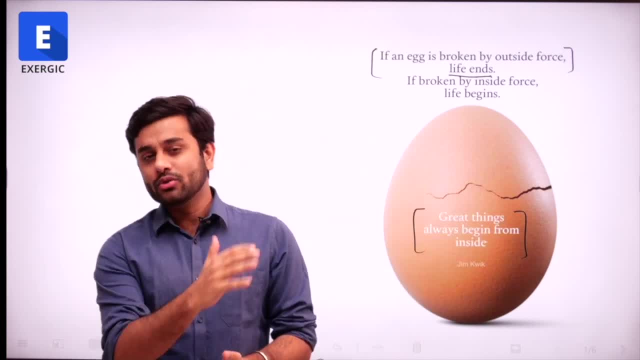 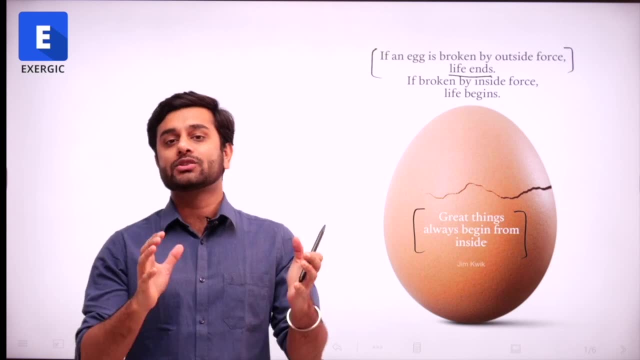 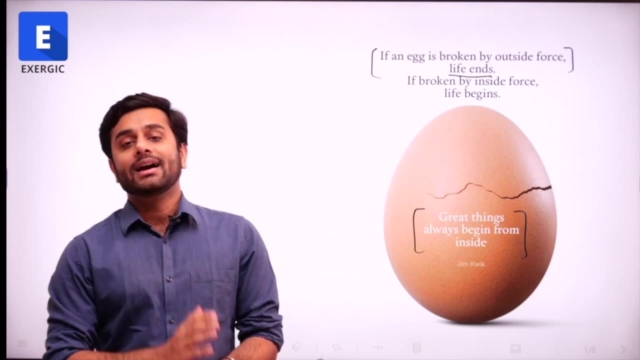 which is unwanted in most of the times, on any given body, on any component, has a negative effect. It tries to break it, crack it, bend it, distort it, deform it. As an engineer, it is your duty to ensure that the external load of the egg is broken by the outside force. If an egg is broken, 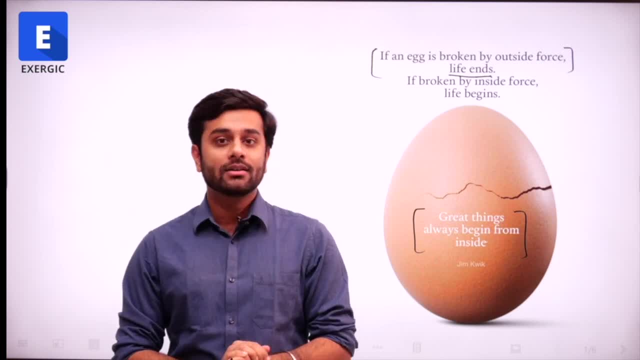 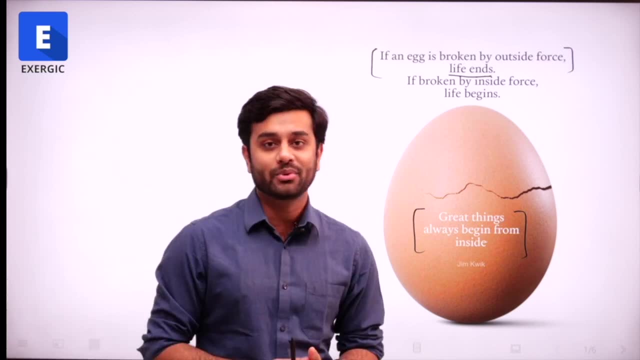 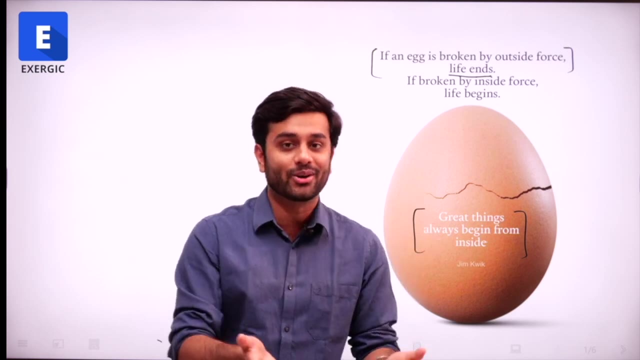 by the outside force, the life ends. Any external load, any external forces are not having a very dangerous effect on the body. In the case of egg, you cannot control it because humans don't manufacture the eggs And, obviously, since you want the egg to get broken from the inside, 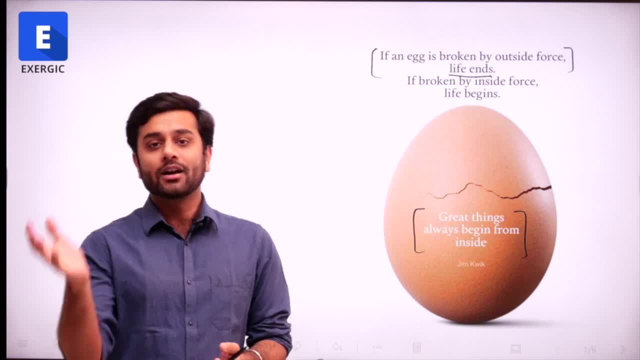 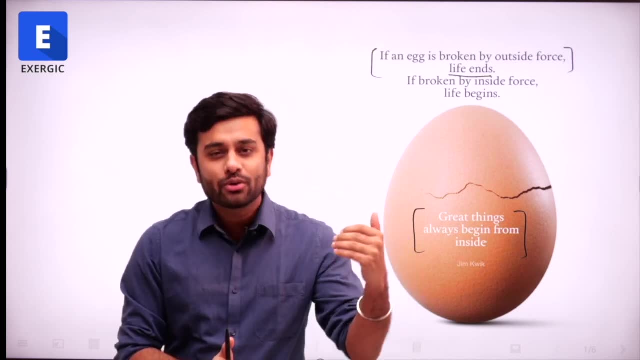 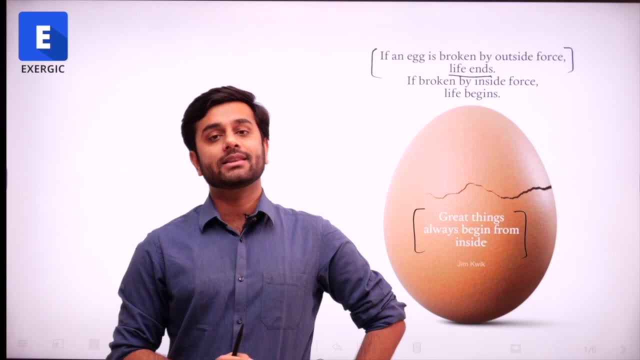 so obviously it is not good that egg is very hard. Coming to the points, coming to the components that we design, that humans design and especially we design them to, you know, be in use for long and long years. We want them to be of such a quality that they don't get bent. 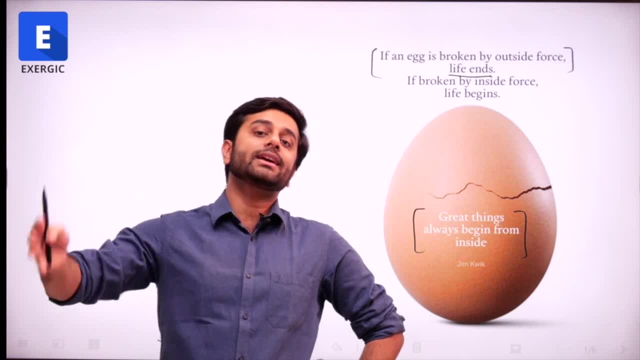 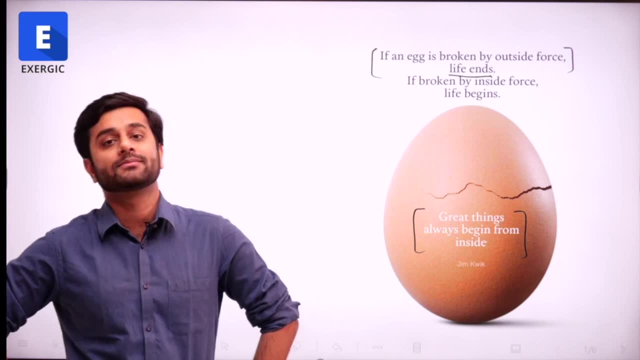 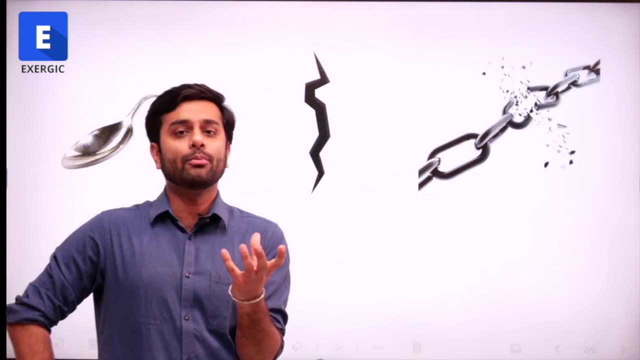 distort, deform due to any external load, any external force that is being applied to them. Right, That is what we are going to study. in strength of materials, There are a variety of things that can go wrong with any component that we have, Any component under use under the action. 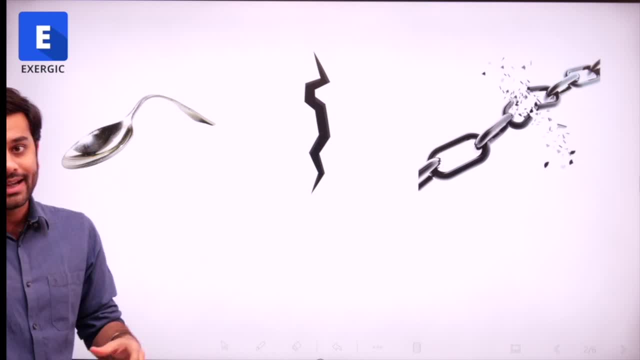 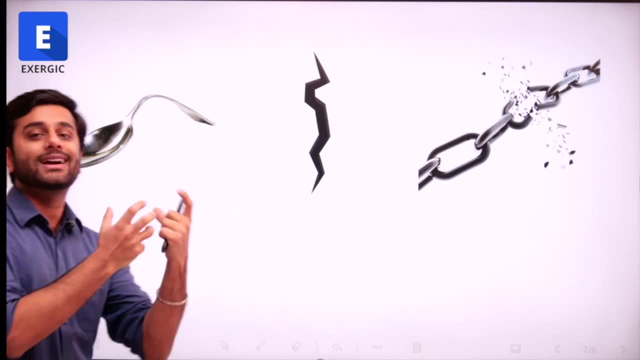 of external force, external load, external force, external force, external load, external force, external load. Either it can get bent right- I have shown you a bent spoon, a very small example I am giving you right now- Or there can be cracks in that particular component, particular material. 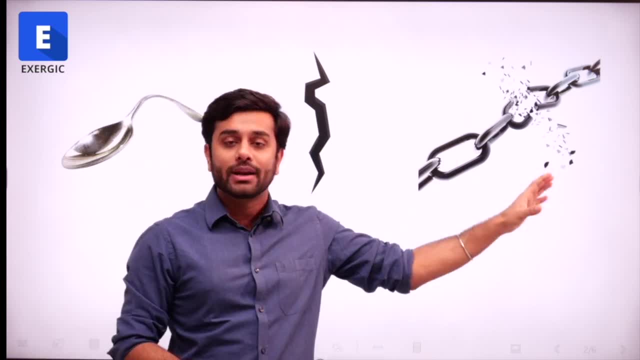 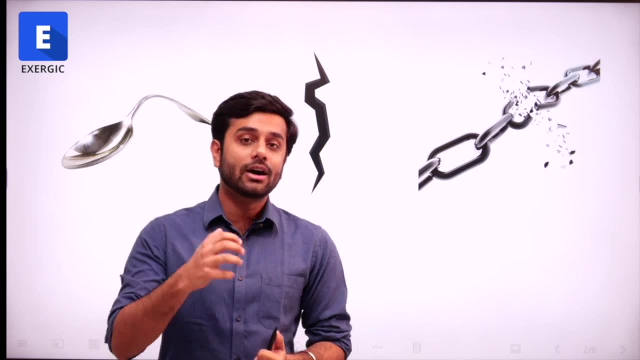 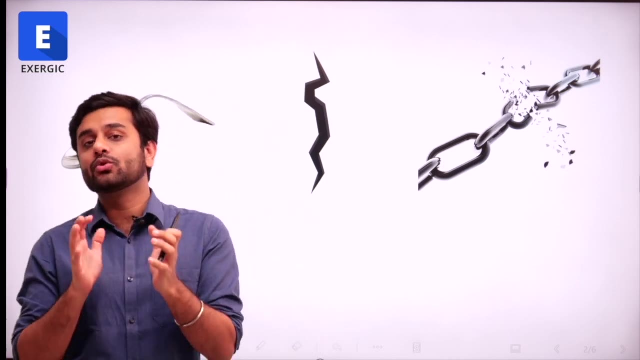 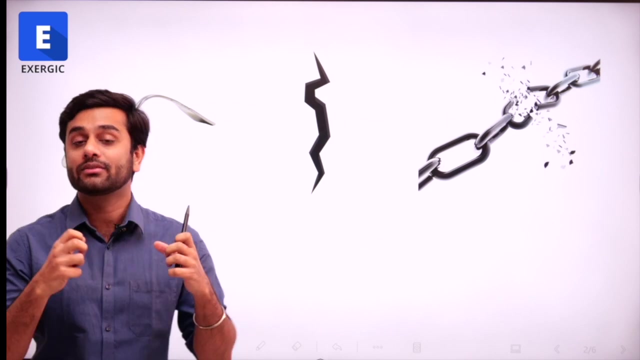 which can propagate, which can increase and finally break that particular component, Right or not. As an engineer, it's your responsibility, it is our responsibility to ensure a design using those materials, those designs, those components that do not bend, crack or fracture or break under the action of external loads, external forces. 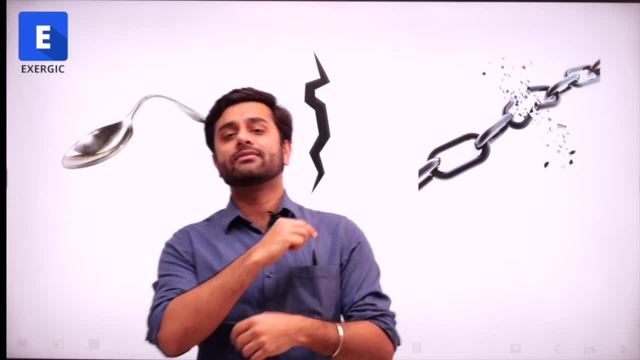 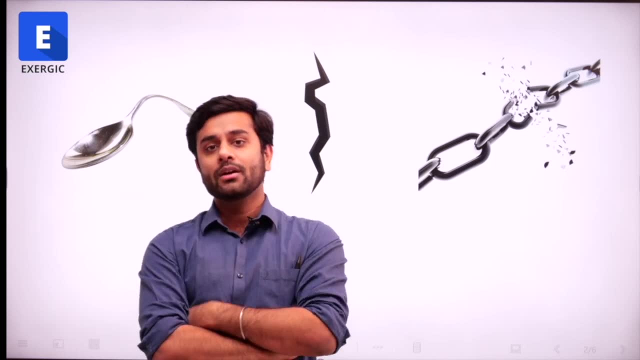 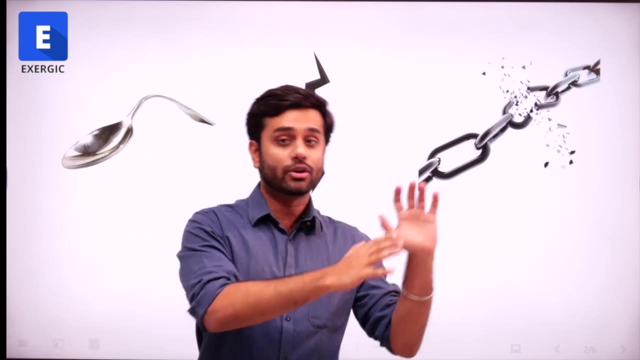 Right, And that is what strength of materials is going to do. It's a very important subject and very interesting subject has a variety of practical applications. Whatever component we have does not matter whether in mechanical engineering or electrical engineering or electronics or computer science engineering. Whatever component you have, it is very much. 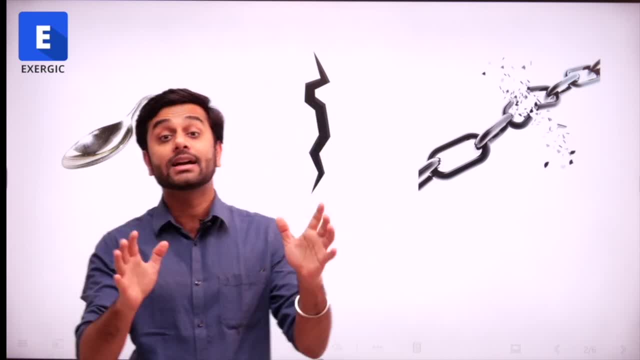 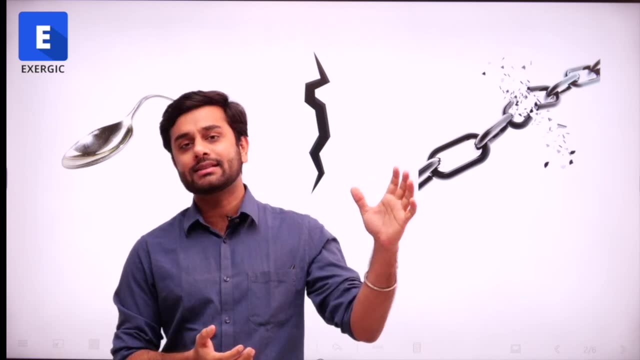 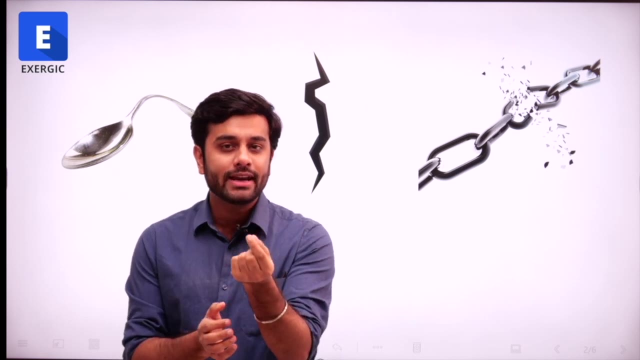 necessary to ensure that it does not break right Physically, does not break, bend, distort right. Otherwise it will be of no use, Whether it's any electronics component, as I told you, or any mechanical component, right Right from a very small needle to a very small iron. 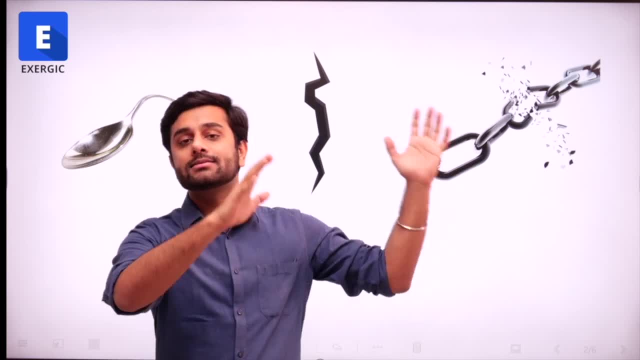 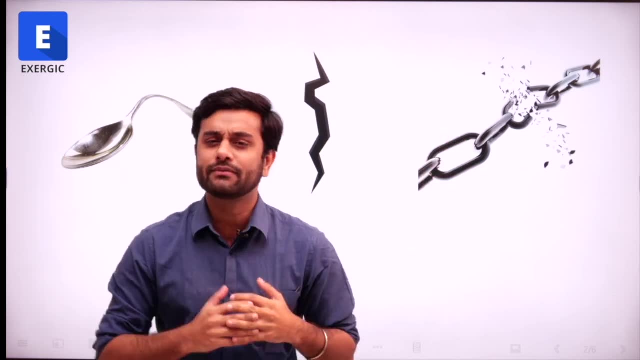 nail to very large ships and buildings and bridges, everything that we design, from that small size to those small spec, like a pannier, like oh-oh wood- I have you have processコl. to those large dimensions, large sizes. everything we want to be in the right shape, right size. 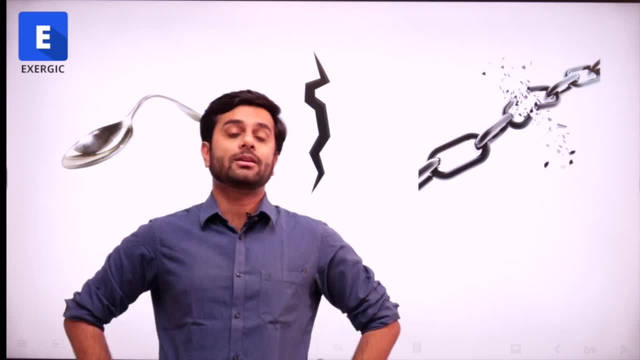 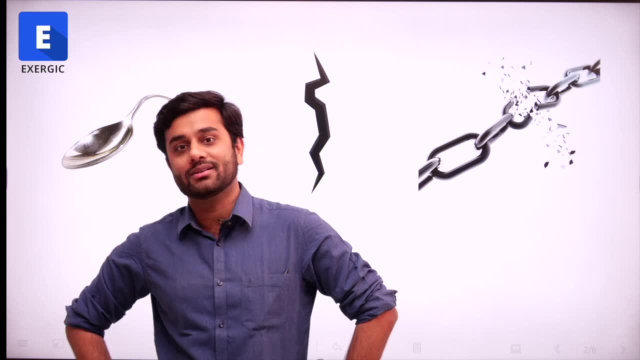 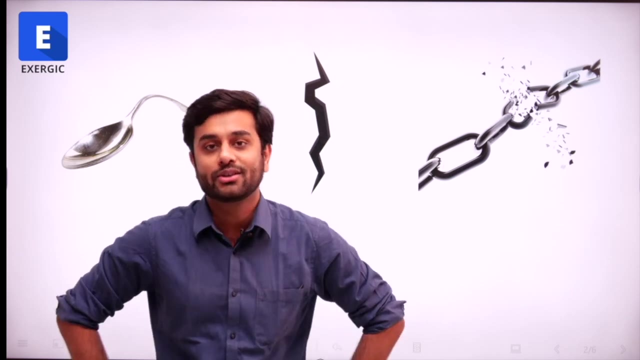 without any distortion, bending and any kind of fracture and breakage right in strength of materials. we are going to study about that and how we can ensure that the loads does not do any negative effect on the body. obviously there will be negative effects. you cannot say that a force 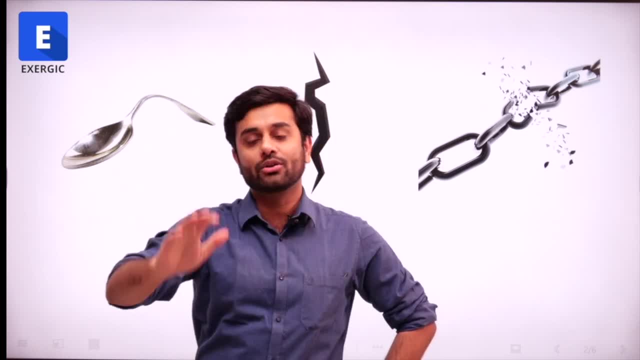 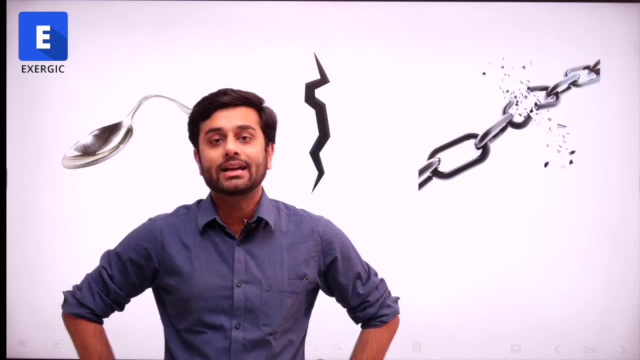 is applied or a load is applied and nothing will happen to the body. you are not god, we are not god, right? but what we can ensure that it does not have a very dangerous effect that will make the component useless. right, that is what we are going to study in detail. okay, in detail we will study. 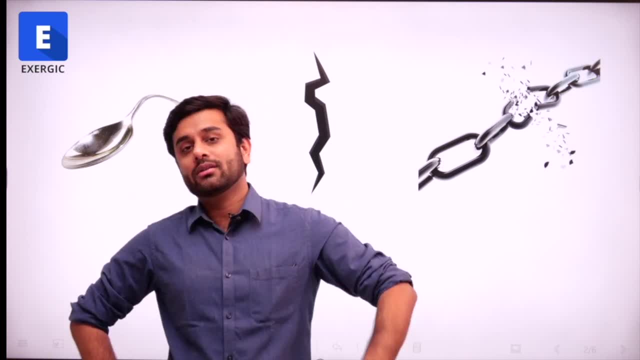 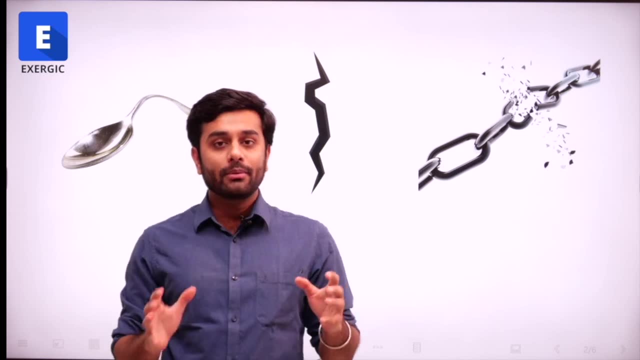 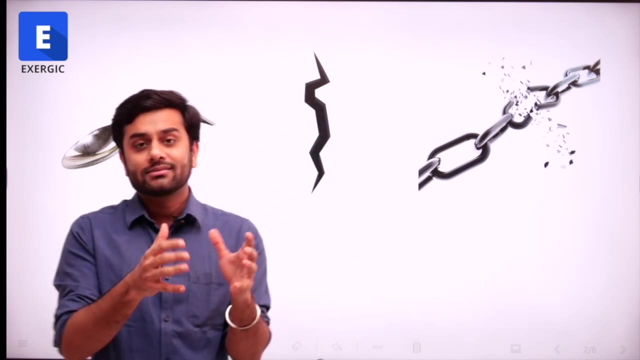 that. but let me tell you, even before we start the discussion, that it's a very intuitive subject. intuitive means you will be able to feel what we are studying. you will be able to, you know, understand what is going on, sometimes without even understanding the concepts, without even totally understanding what is going on you. 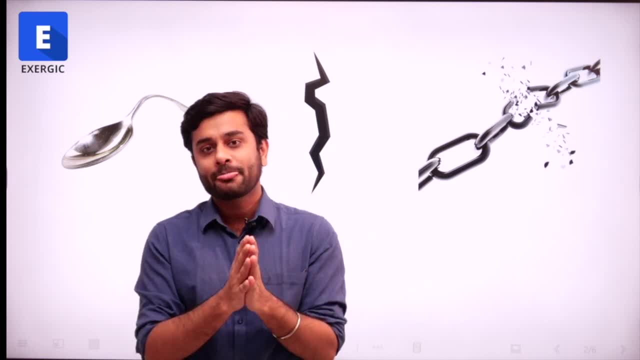 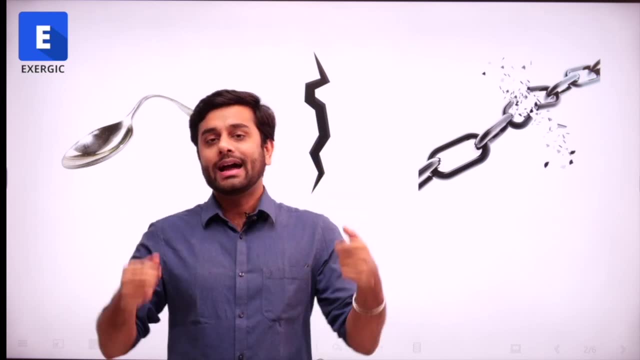 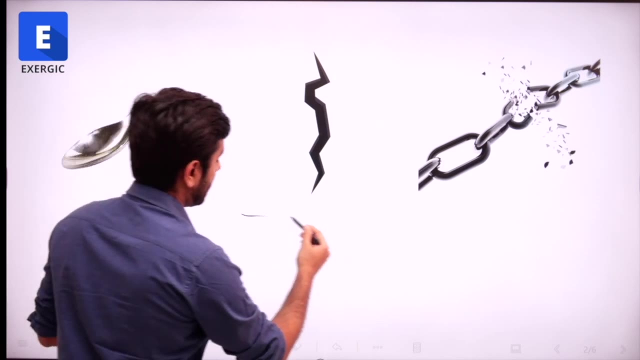 can feel that what is going to happen? for example, if there is a thread, okay, a thread, a string cord, small, thin cord, thin string and other cord is thicker, right, one small thread, a very thin thread, and another thread we have which is thicker, okay, and what we are going to do now that we are going 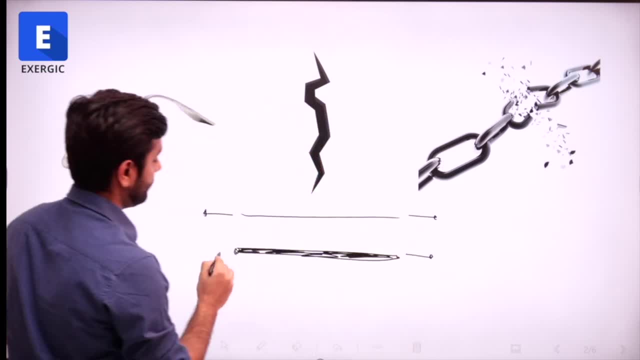 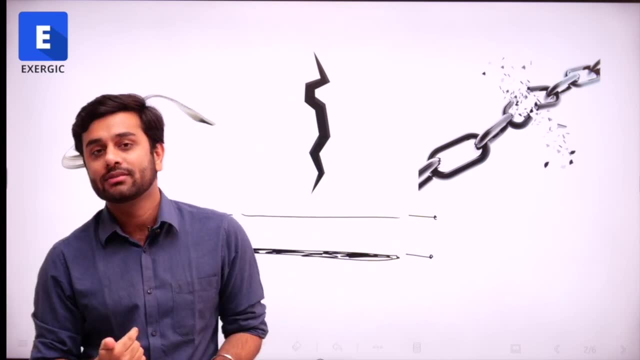 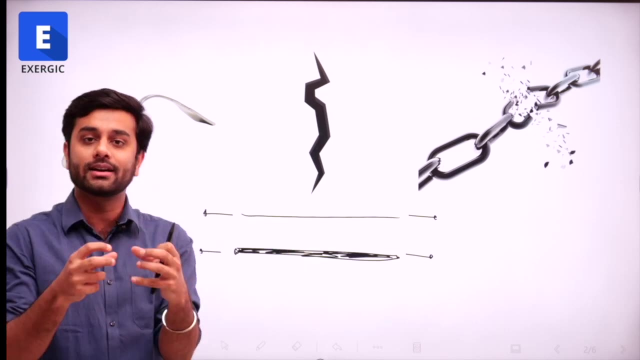 to apply a force on these threads. right, we are going to. you know, extend it. try to extend it. if one of them breaks, tell me which one is it going to be. if i am applying the same force on two threads- one is thinner, other is thicker- of the same material and one of them is going to break, tell me which one. 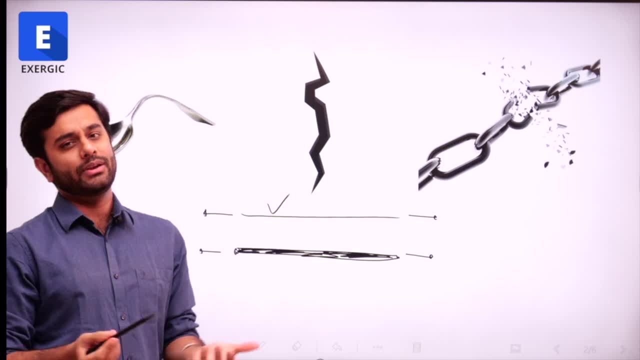 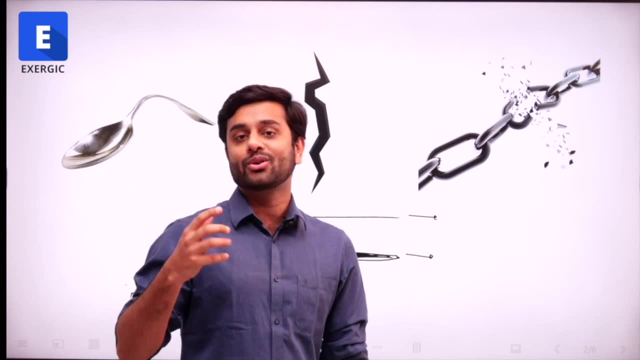 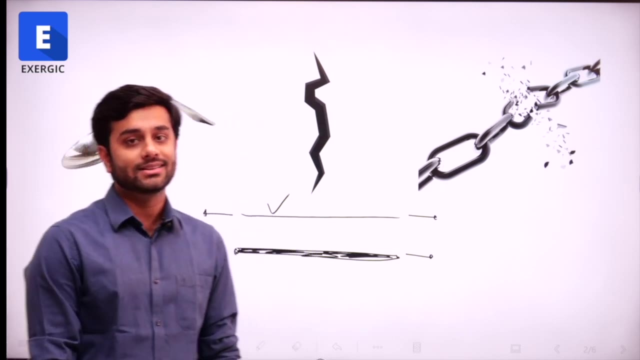 will break first. this is going to break first right. very clear. it's a thin one. if i start asking you why, you might not be able to conceptually answer it correctly at this point of time, but intuitively you can feel that this is the one which will break first. similarly, i will give you 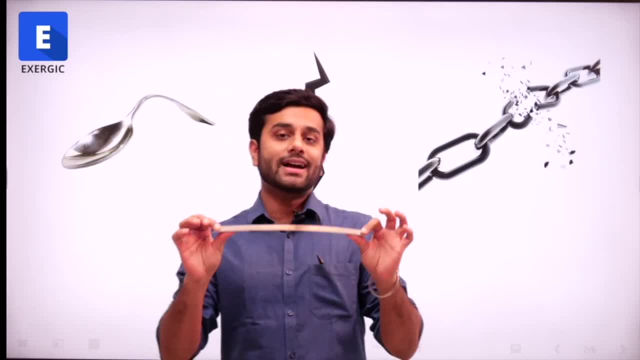 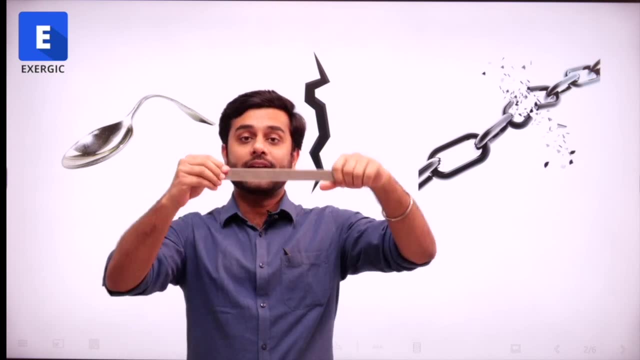 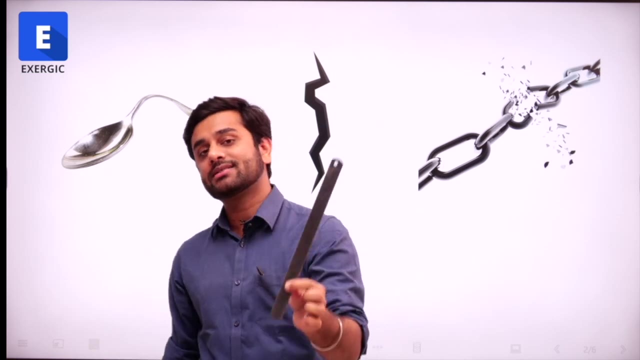 one more example at this point of time. now suppose i have this scale, this ruler, right? if i try to bend it like this and if i try to bend it like this, tell me which one of them will bend? even without having a scale, you can answer based upon intuitive feelings. this is a scale. if i try. 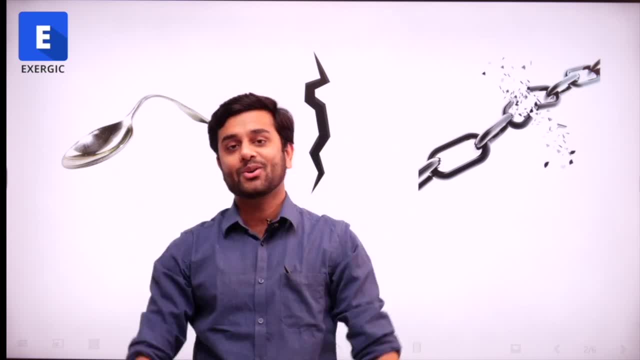 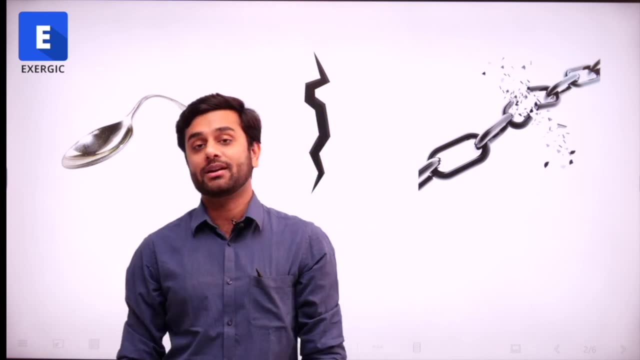 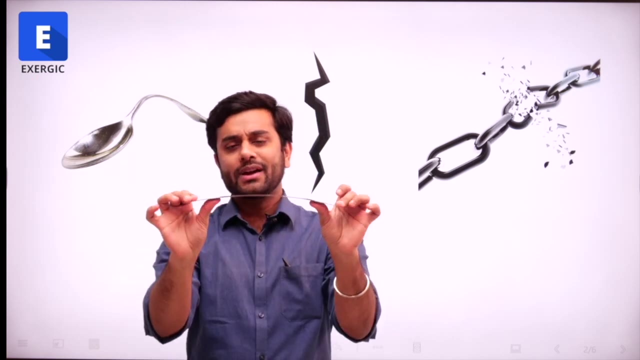 to bend it like this, like this, or if i try to bend it like this, like this, what do you think which one of them will be easier to bend? very easily, you can answer this if you intuitively feel what is going on right. very easy to bend it like this, but if you try to bend it like this, it's not easy. it's. 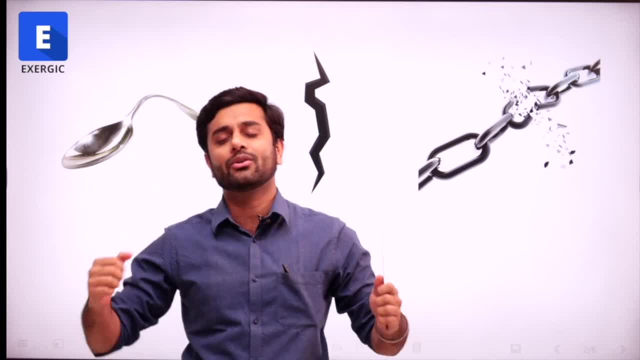 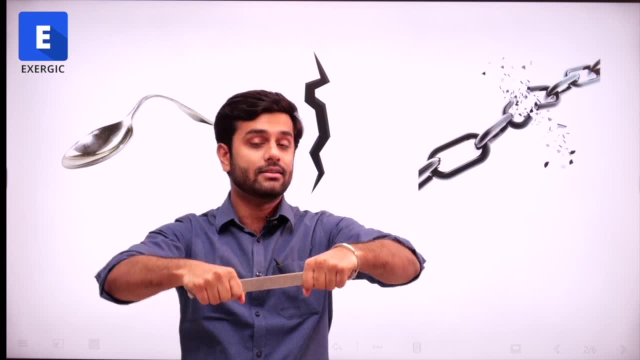 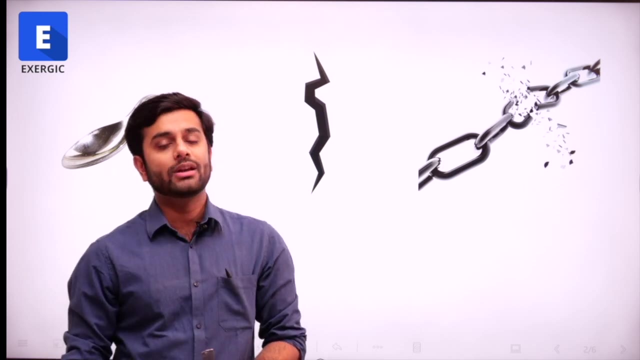 not having a scale in your hand. if you just close your eyes and imagine a scale or any such a flat surface, you will realize that it's easy to bend it like this, but it's not easy to bend it like this right, this is an experiment, right which the conclusion of this experiment, you can very easily 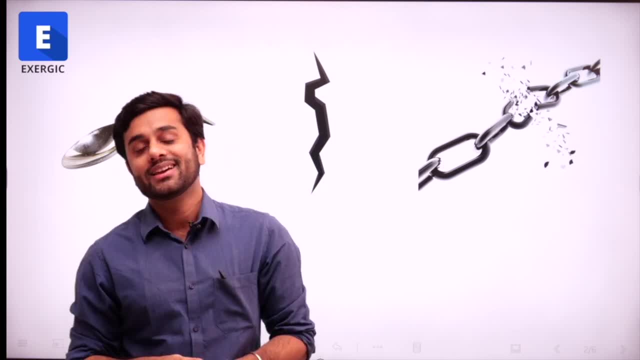 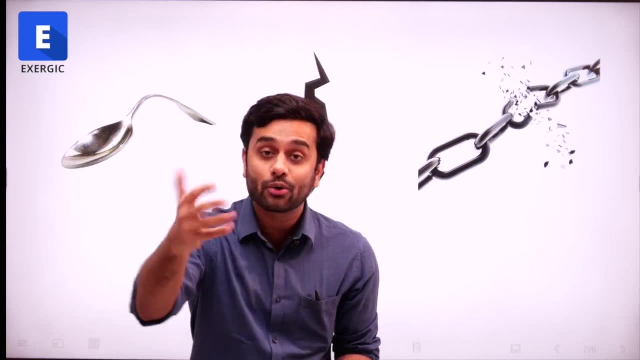 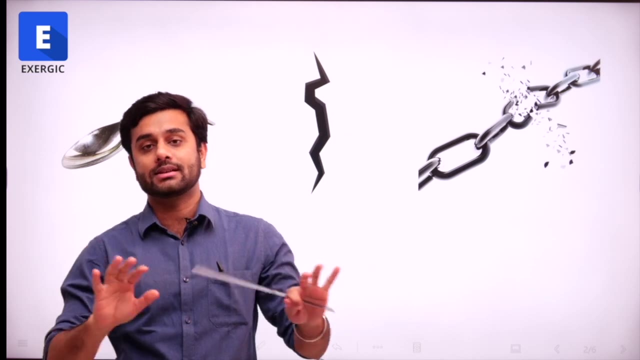 you know, predict without even knowing the concept. if i asked you same thing for a different system, for some electrical system, and i asked you the conclusion of that experiment, you might not be able to answer it without knowing the concept. right at this point of time we have not discussed why is it able to easily bend in like this, but it's not able to. 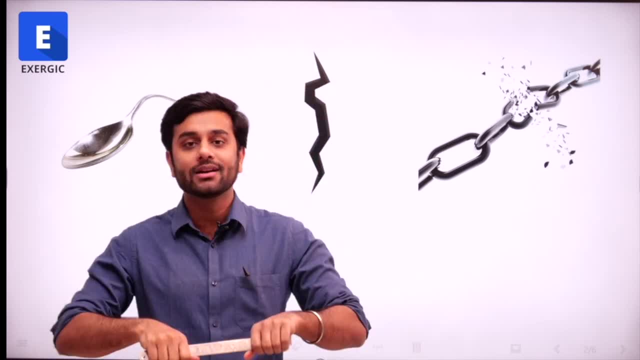 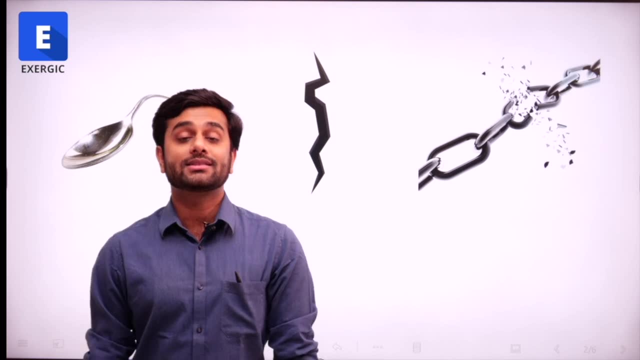 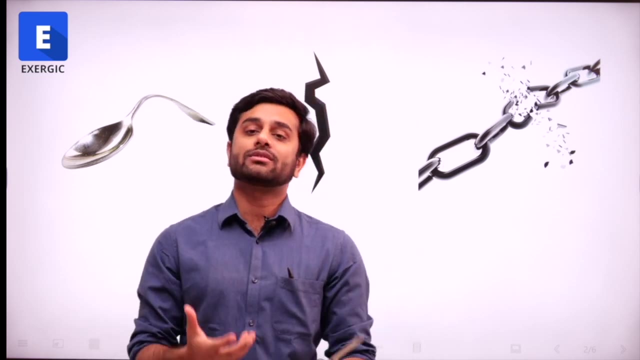 bend like this. material is same right. the applied moment, applied load is also same. but how is it happening? what concepts are governing this? we have not discussed yet, but still we are in a state to predict the conclusion of this experiment. it's the intuitiveness of strength of materials and not 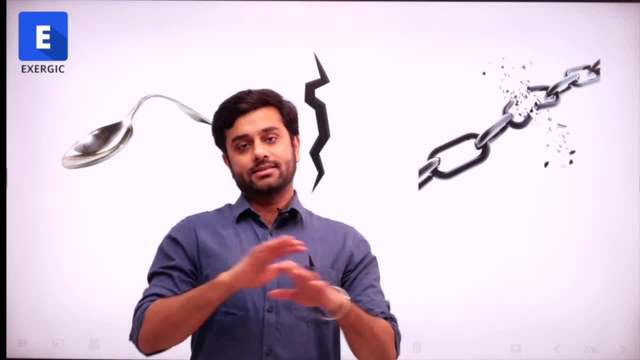 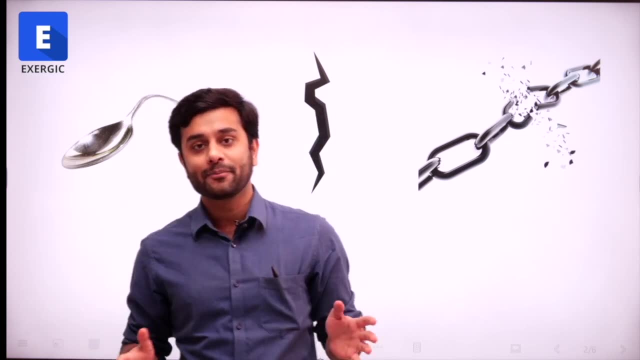 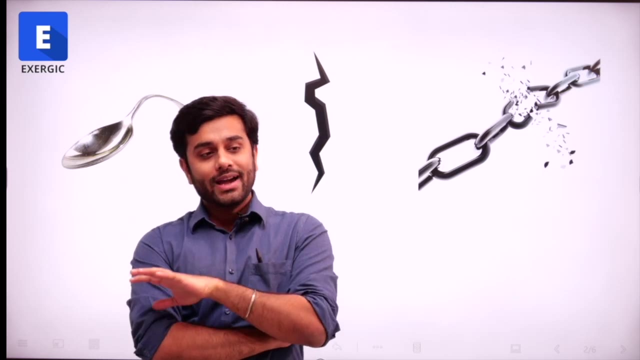 only strength of materials. this is so much more than the strength of materials. it's the strength of materials being one of those, so it makes the subject very interesting. once we are going to cover different concepts of strength of materials, you will realize that why things are designed and 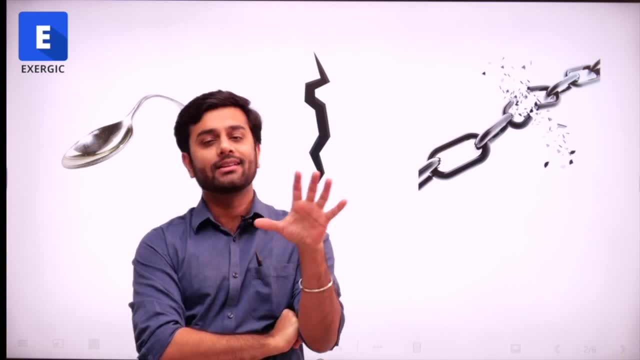 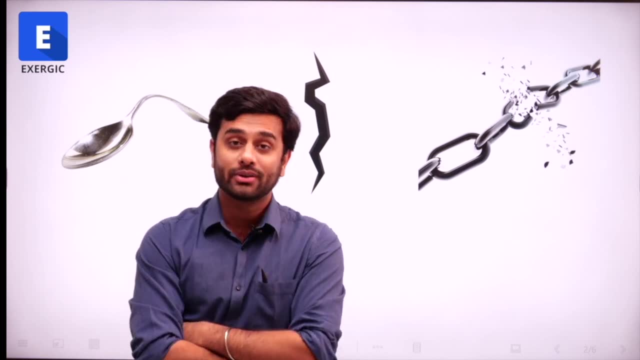 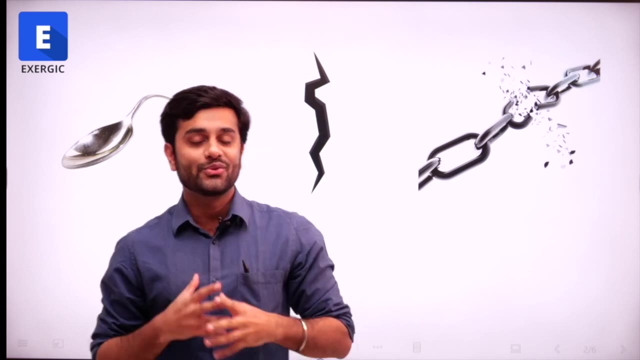 made the way they are, you will start realizing it. whether it's a small table, small chair, or any door or big bridges, you will be able to understand that, why they are designed and made the way they are made in that particular shape, what factors, concepts work behind them. you will start getting. 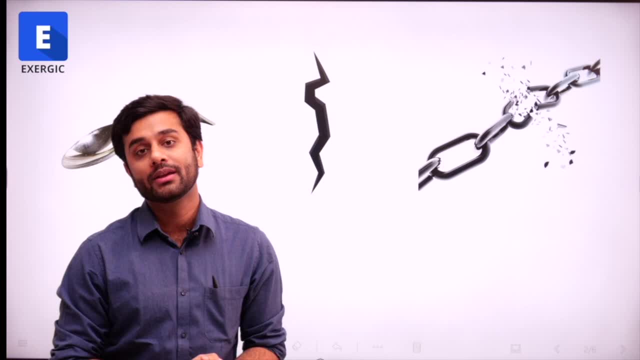 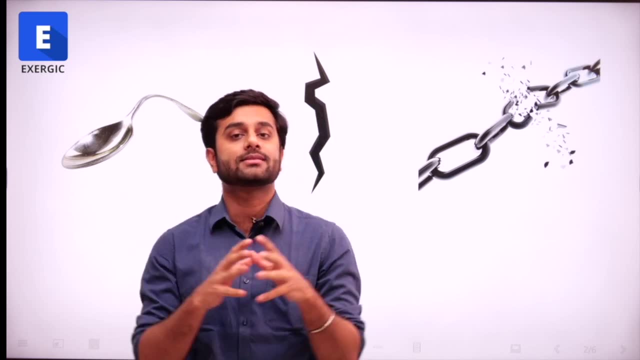 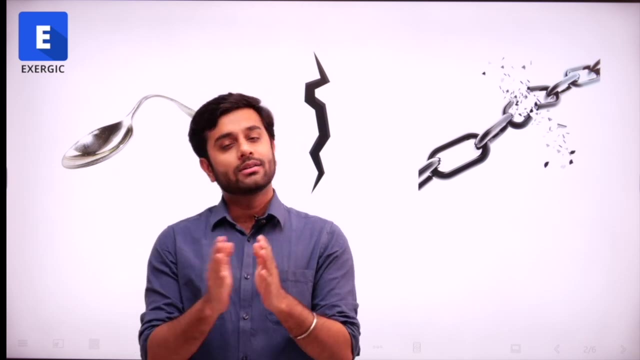 a feel of that. so it's a very interesting subject. if i talk about from the point of view of gate, again, it's very much important. it's one of the fundamental subjects of mechanical engineering, as well as civil engineering. in terms of marks or weightage, if i tell you, the range keeps on. 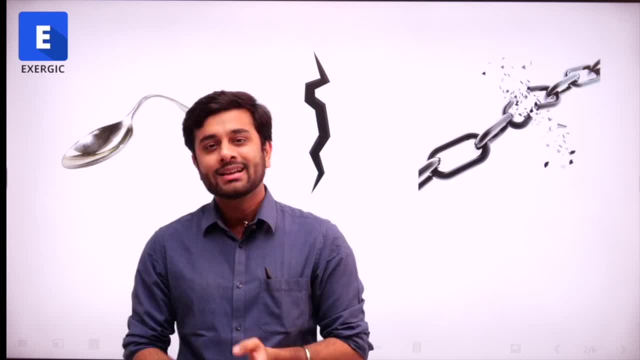 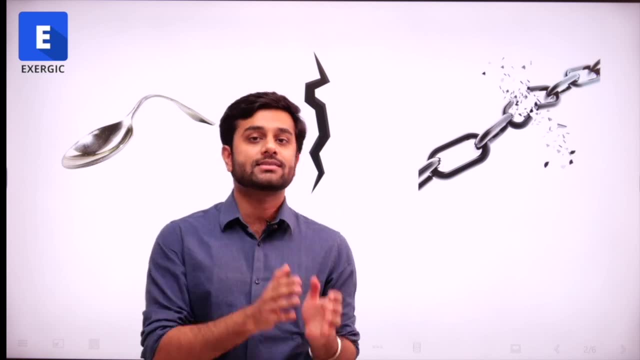 changing depending upon the year, depending upon the set. general range is from seven marks to ten marks every year. as i told you, it can change. it depends upon which year and which set you are going to get. but that's not the point here. the point is that the concepts that we are going to 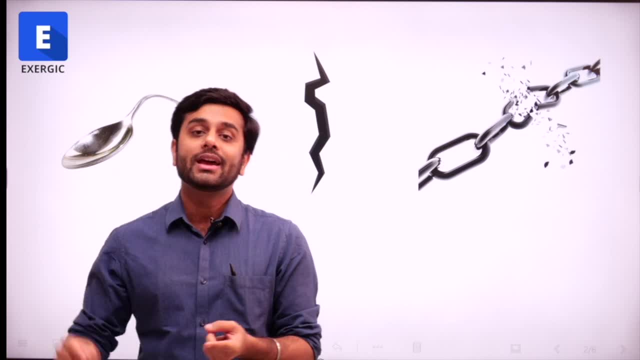 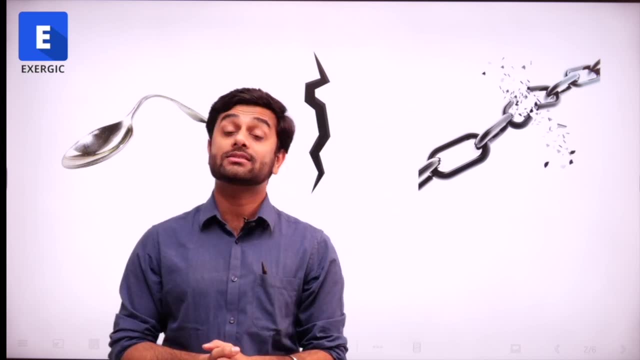 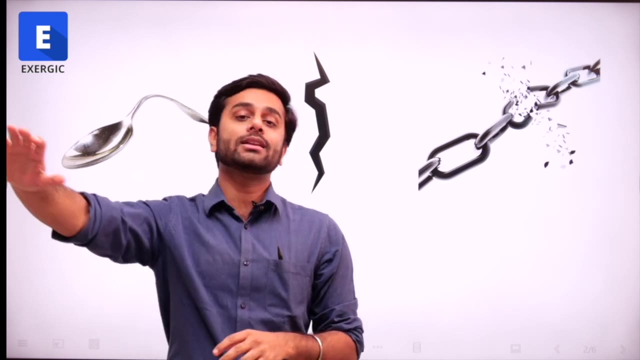 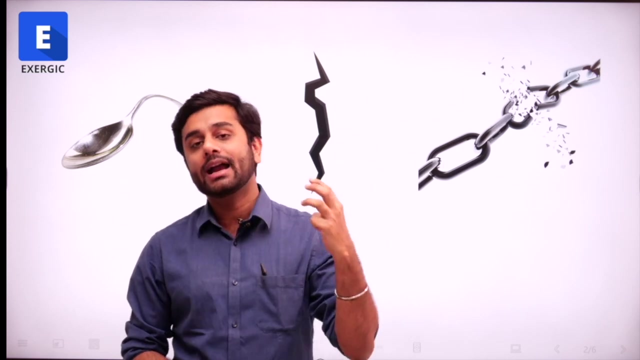 study in strength of materials are going to be used in fluid mechanics, also in machine design, also to some extent in manufacturing and production subject as well. so it is a very fundamental subject of mechanical engineering. without totally understanding the concepts of strength of materials you won't understand and enjoy fluid mechanics, machine design and manufacturing. and 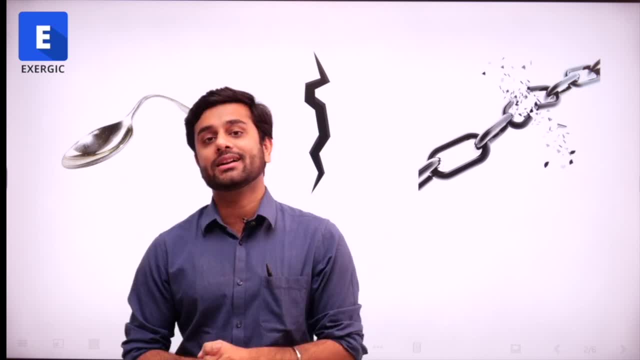 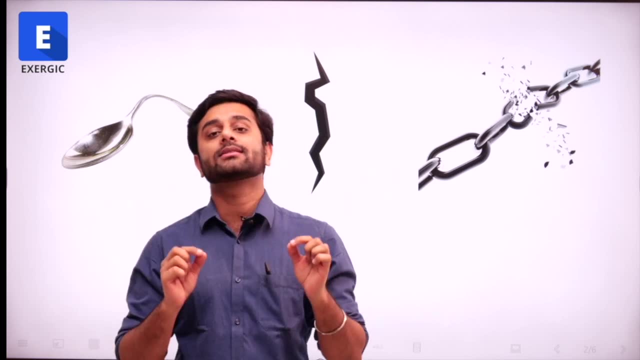 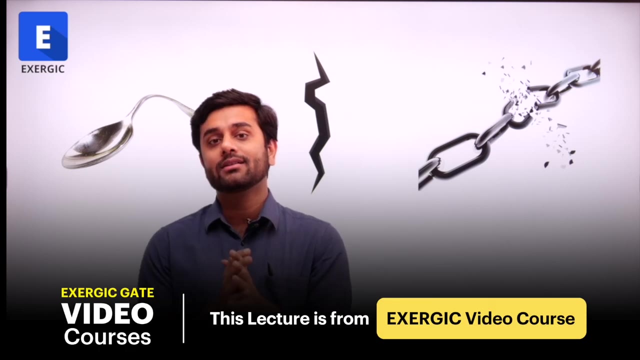 production. that much so. this subject, undoubtedly, is extremely important. i want your undivided attention when i am teaching this subject- for any other subject also, it is true, but this one being one of the most important ones, fundamentally, conceptually, i want a proper undivided attention. 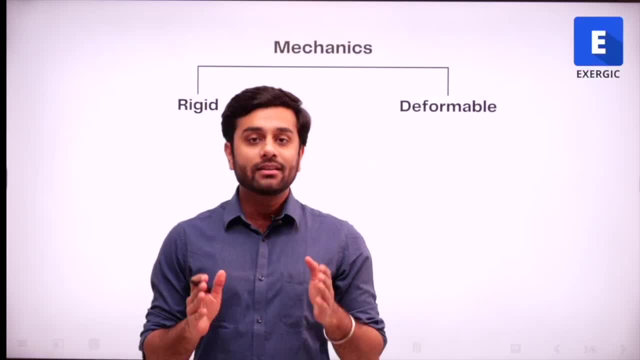 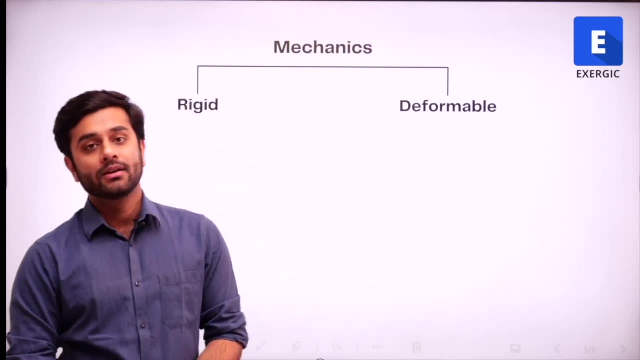 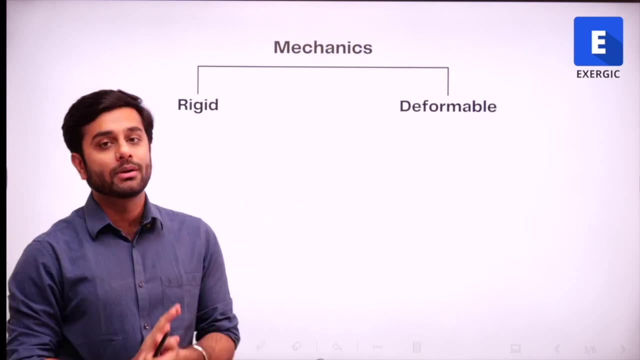 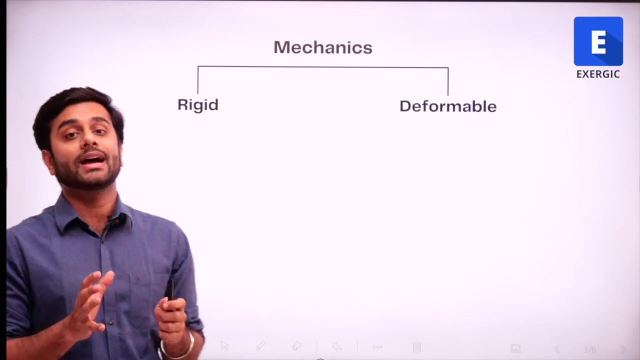 from your end. now, mechanics is a general name, a general branch of study which is divided across many classifications. right, the very first and basic classification of mechanics is between rigid and deformable bodies, whether the body that we are analyzing is it a rigid body or a deformable body. on the basis of that, the first classification is done, and then it branches. 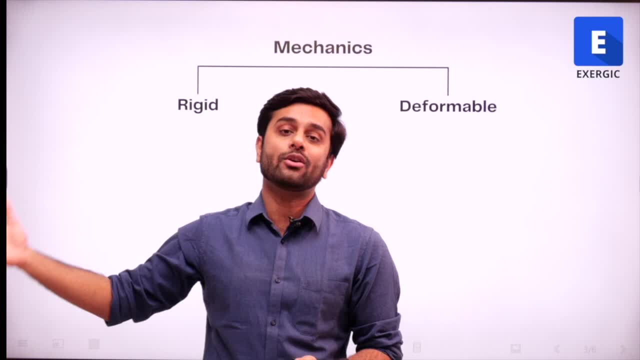 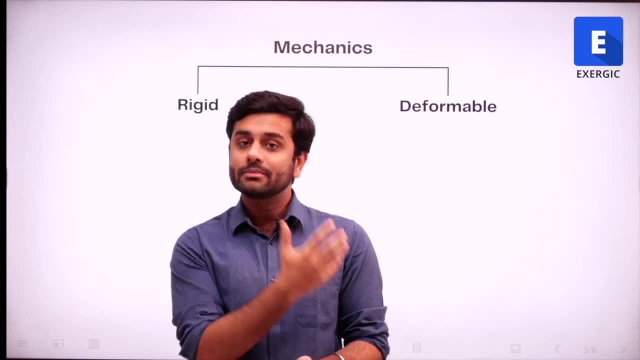 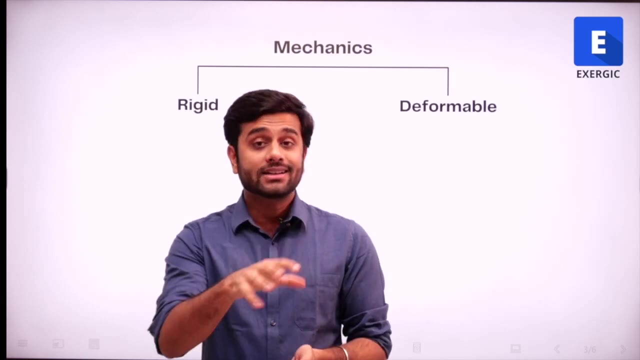 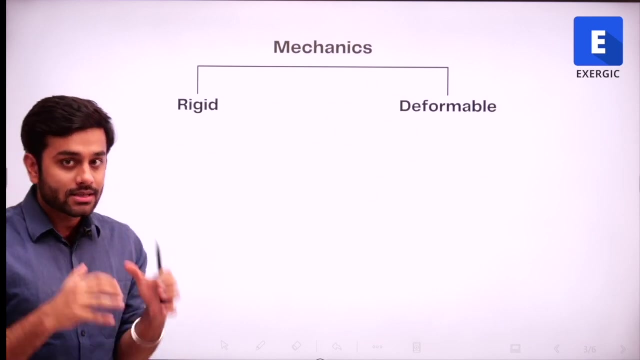 into engineering mechanics, something that we have covered already. right, strength of materials or mechanics of materials is also a mechanics right: fluid mechanics and even theory of machines and vibrations to a great extent. so that classification is what we are going to study now. so the first classification, as i told you, is based upon whether the body that we are considering is a rigid body. 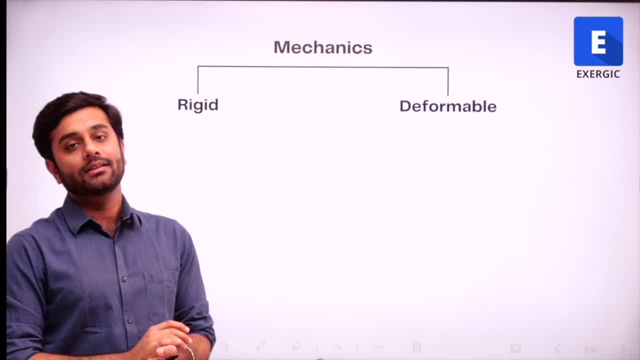 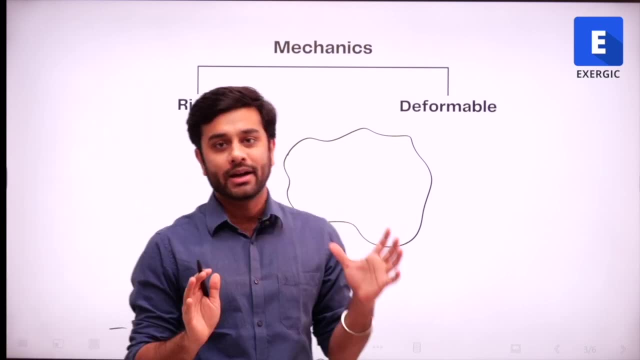 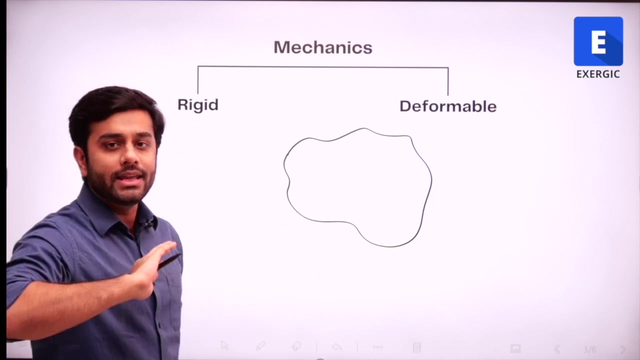 let us first understand what exactly is meant by a rigid body or a deformable body. suppose you have a general body shape i have shown here. right, it's a general solid body that i have shown here. on this body, any point, any two points, you take any two points. it can be this one, this one or this one. 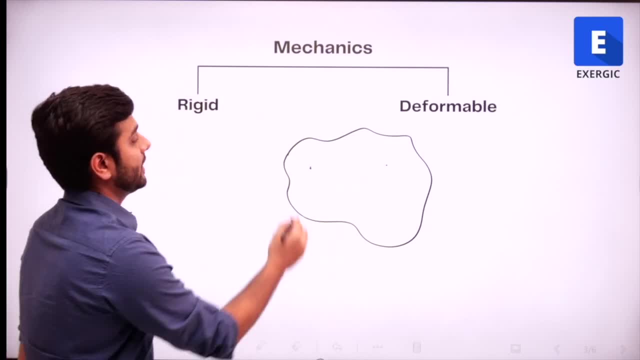 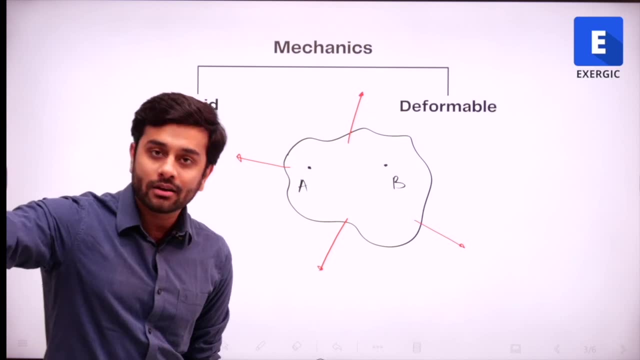 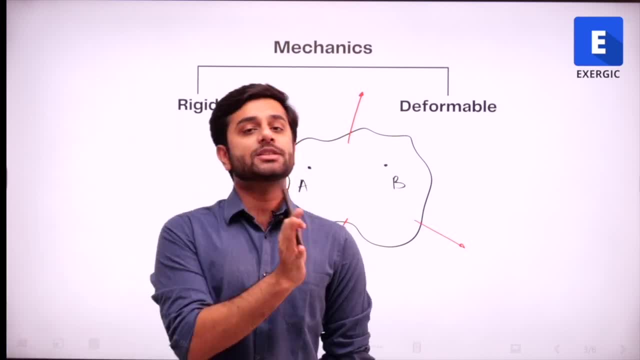 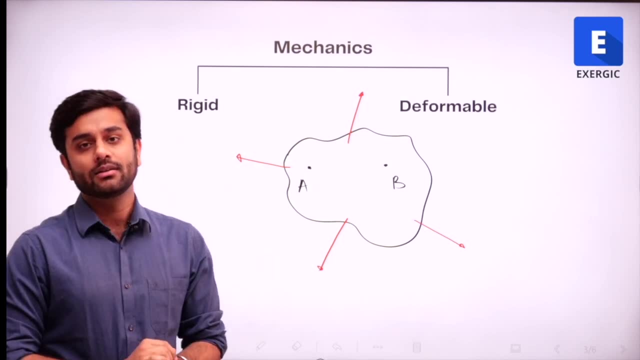 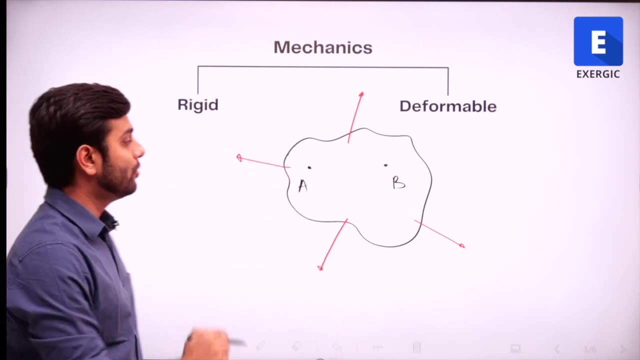 that in any general case, it is very much possible that the shape of this body is going to change or the size of this body is going to change, right? I'm sure you know the difference between shape and size. it's very important. it's a basic English term, but you must know and realize the difference between shape and 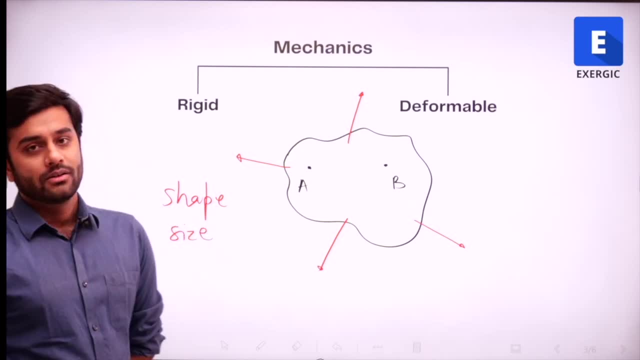 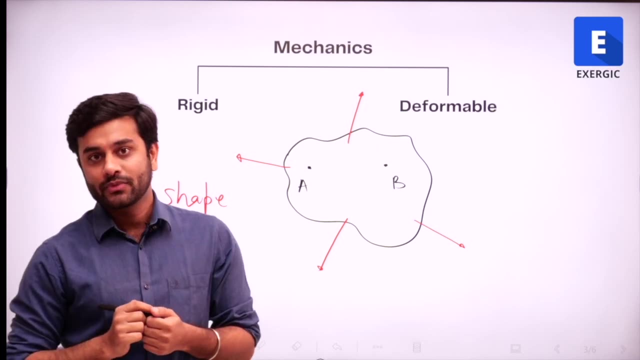 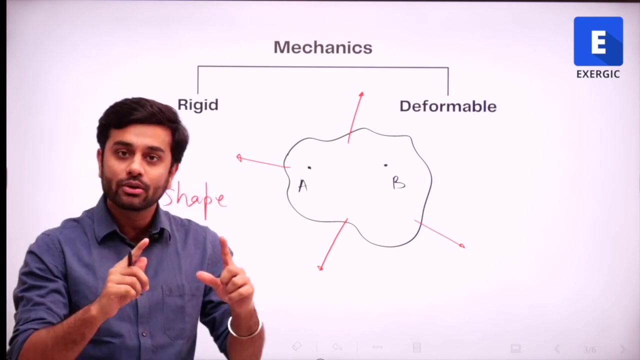 size. shape is something which tells you how the body looks from. you know the external point of view. what I mean to say? that if the body looks cuboidal in shape, if it looks spherical in shape, if it looks triangular in shape, right, these all are the shapes of the body. it defines the orientation, or defines. 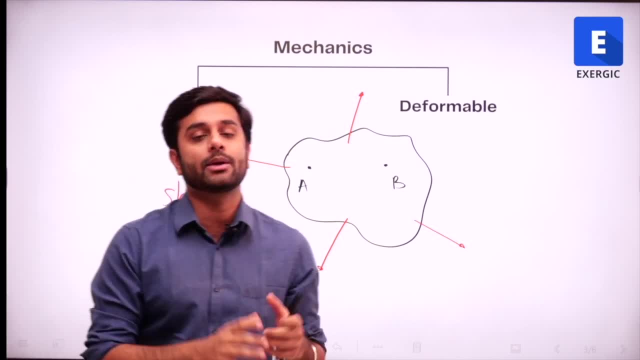 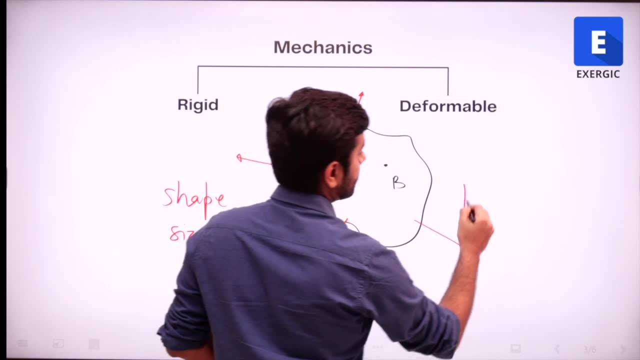 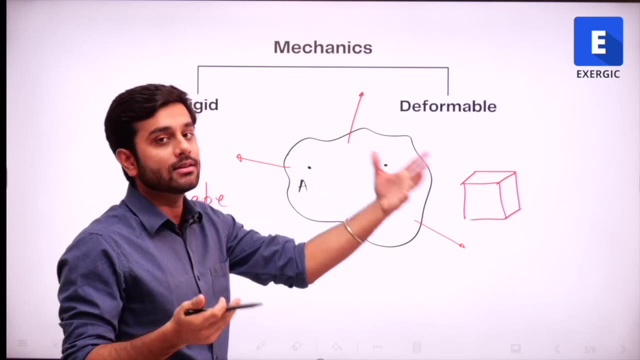 exterior, exterior look of the body. that is called a shape. size refers to how large or how small the body is, and size refers to how large or how small the body is right. so if I tell you through an example, this is a cube which is smaller in size, but the shape is a cube. if I draw another cube, this is also a cube. 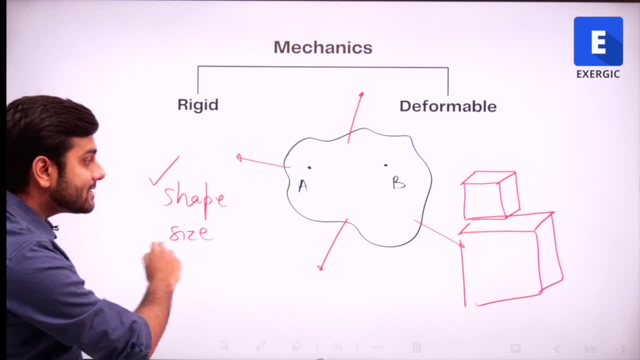 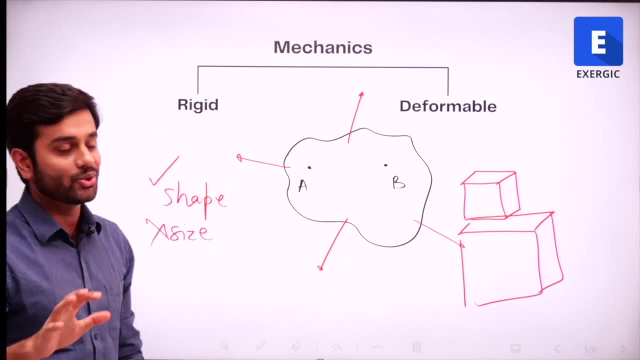 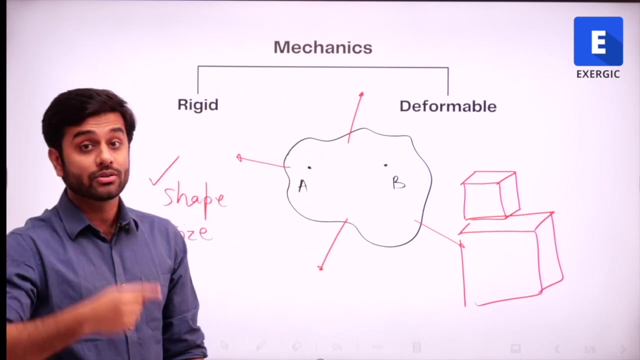 both of them are having the same shape, but their sizes are not same. it is smaller in size, it is larger in size. it's a basic difference. I know strength of materials is not to tell these basic things, but I assume some of you might be having any confusion about them, so I cleared it here because it will be. 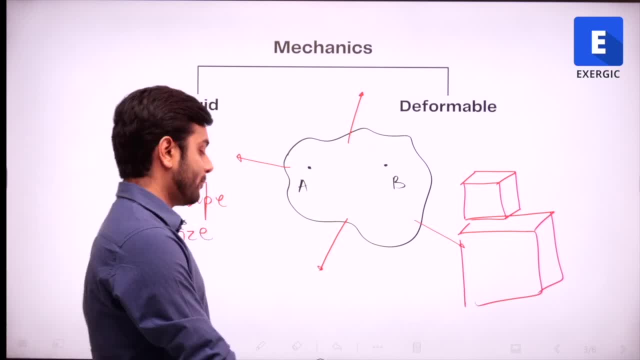 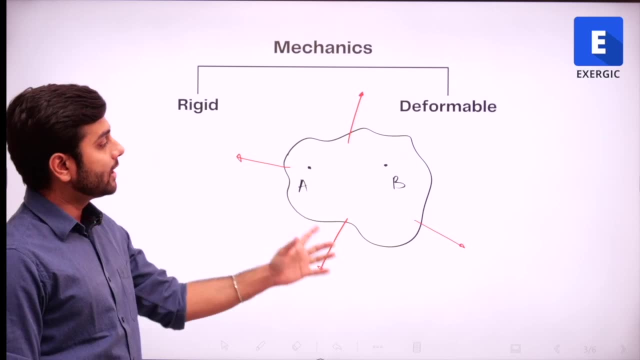 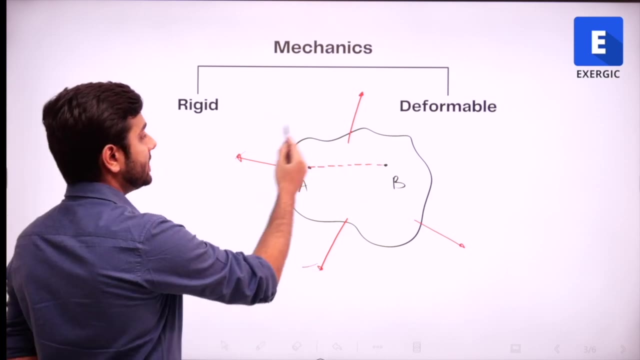 discussed in further discussion of strength of materials. so, coming to the point that we are having a body here- as I can, as you can see here- and this body is acted upon by different external loads of force. now, it is very much possible that, under the action of these forces which are acting on the body, the 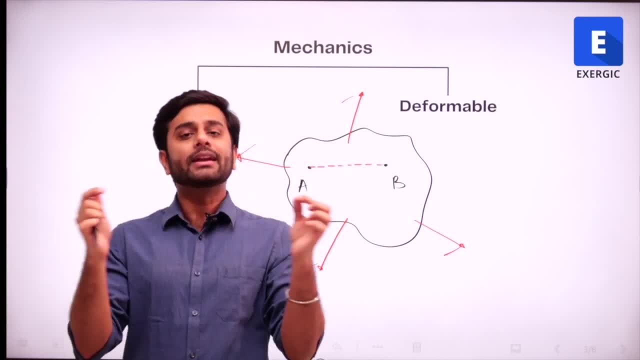 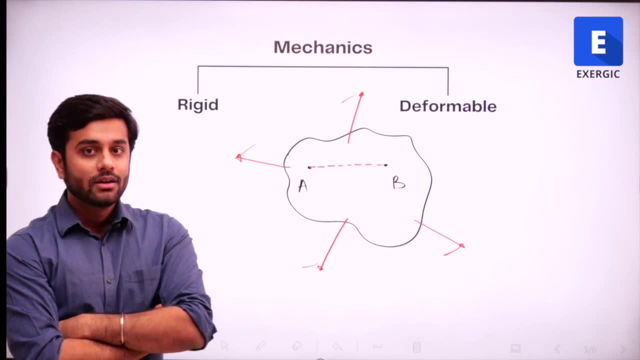 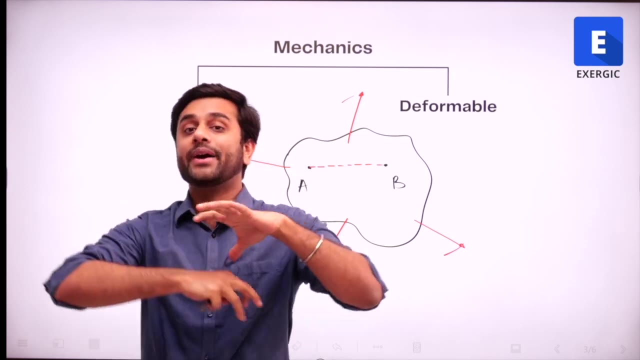 distance between point A and B will change. it can increase, it can decrease. right, a lot of things can happen. a body, a hypothetical body, in which the distance between the points A and B does not change, no matter how many forces you apply, how heavy or how large loads you. 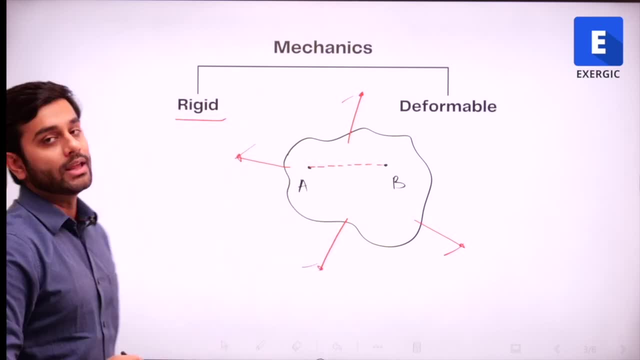 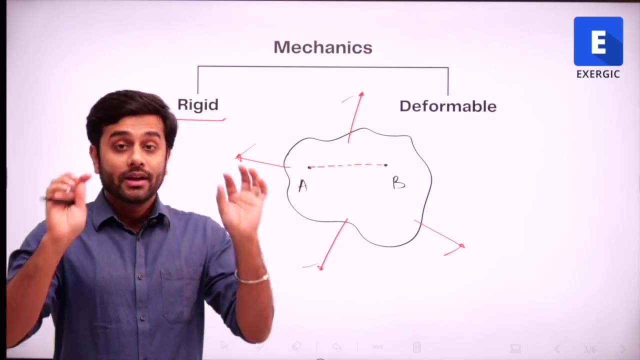 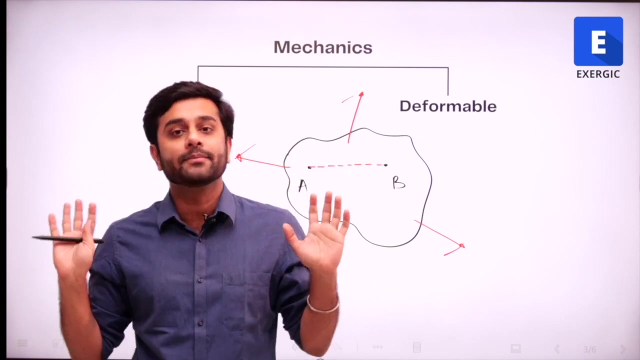 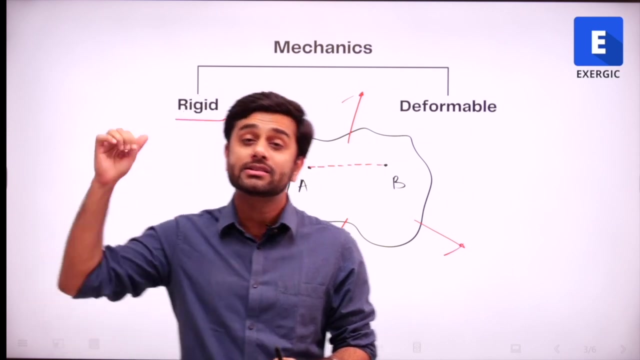 apply, such a body is called as a rigid body. in a rigid body, the distance between any two randomly picked points will not change, irrespective of the external loads or forces applied on that body. obviously this is a hypothetical body. nobody in the world is a perfectly rigid body, because we know that larger the force you apply more. 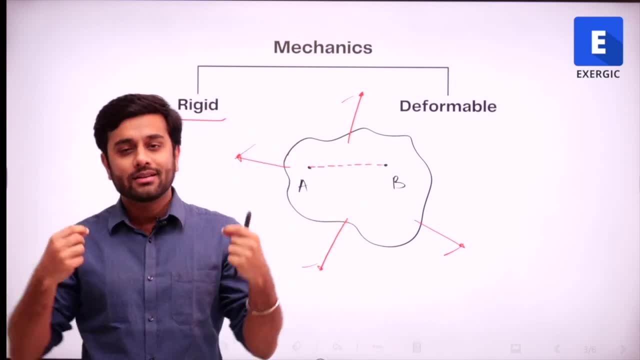 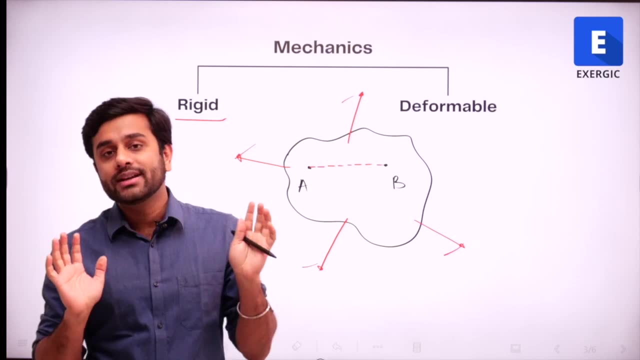 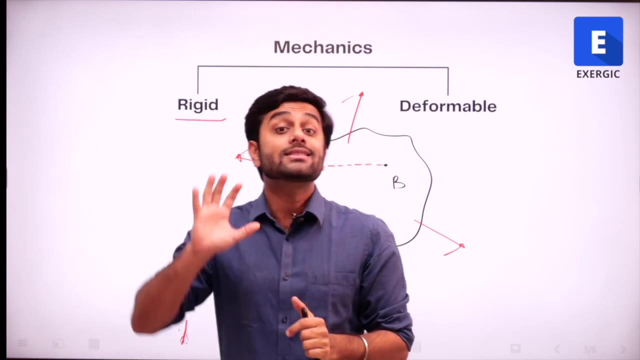 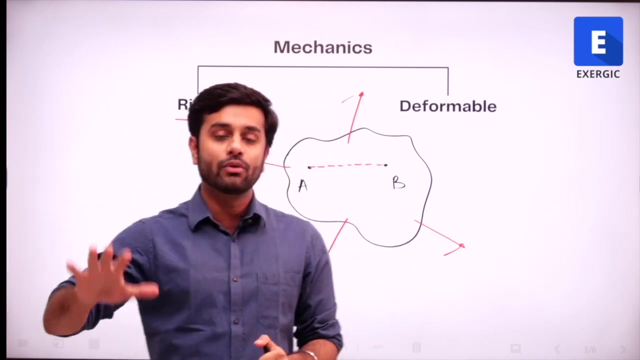 forces are going to act towards the same target. the result will be visible, right, it may not be visible to the naked eye, but the distance between the two points will start to change, will start to increase or decrease, right, but rigid body. body is a not ideal, is a hypothetical body, which means it is not real, no body in the entire world. 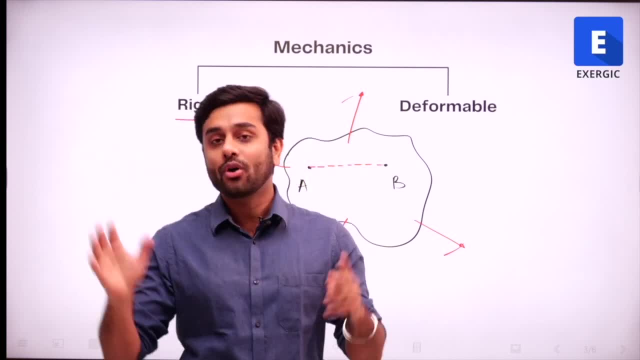 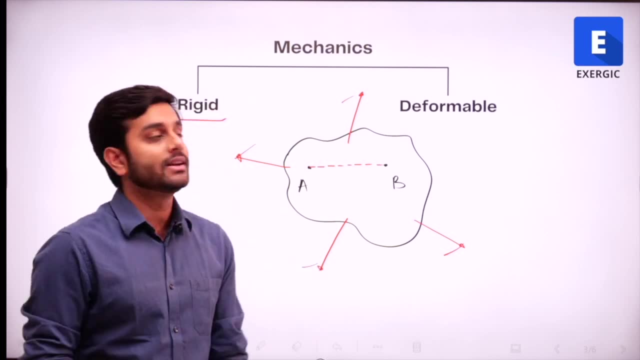 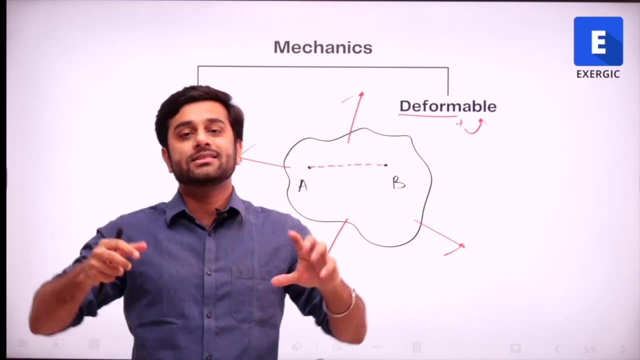 is actually rigid. all the bodies that are available are deformable bodies. what is meant by deformable body? the name itself tells you: deform plus able. a body which is able to get deformed, which can change its shape, its size. right, such a body is called as a deformable body. 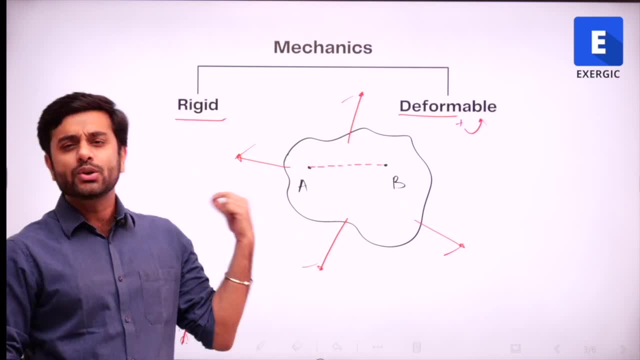 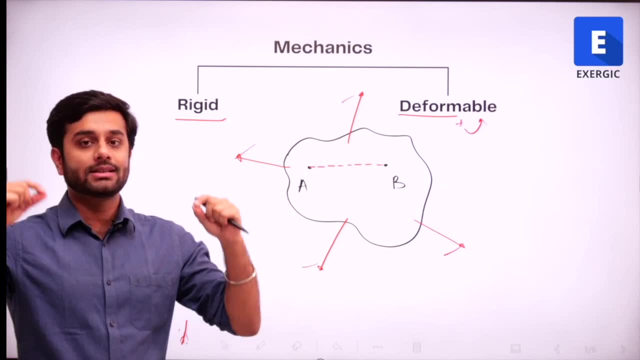 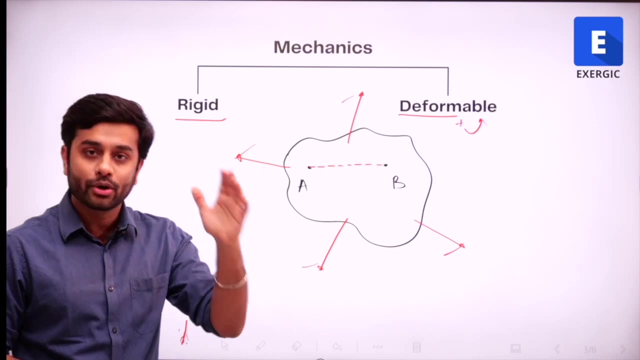 in more technical or conceptual words, any two random points you pick on the body and under the action of applied loads, the distance between those two points will change. such a body is called as a deformable body. all real bodies are deformable. so after understanding the first classification, 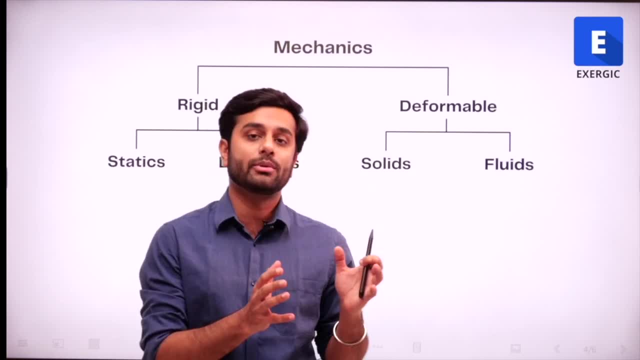 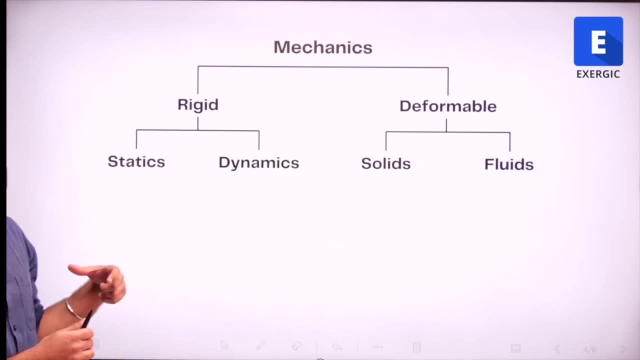 on the basis of whether the body is deformed or not. the body is deformed or not. the body is deformed or not. the body is rigid or deformable. let us see further classification of it, as you can see that rigid bodies are further divided into two different branch of study. first is statics. 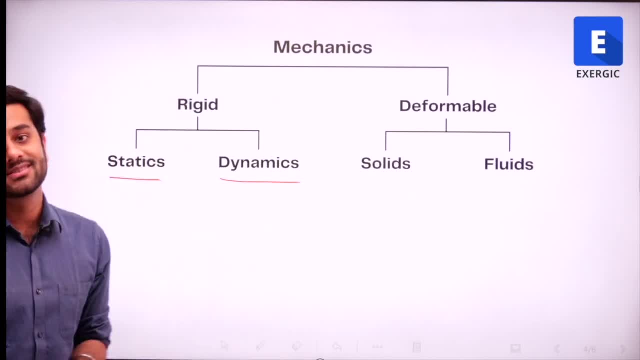 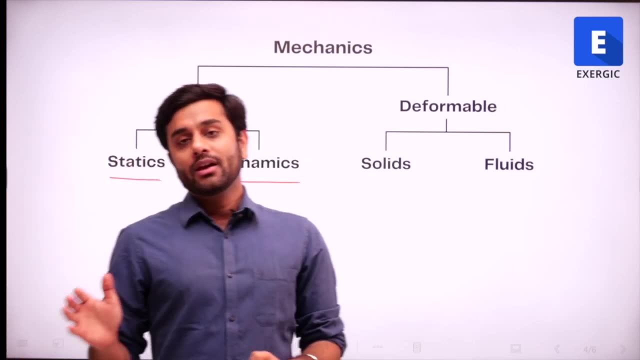 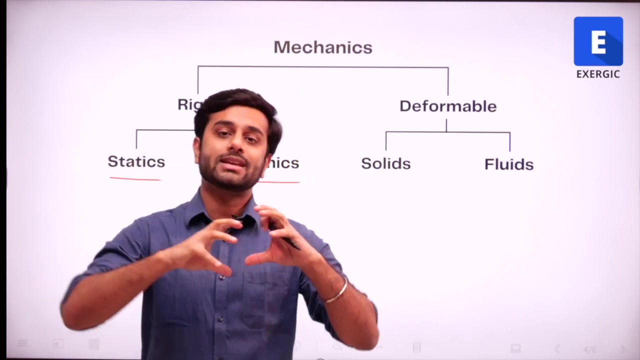 other is dynamics. let me brief you about this, although you already have an idea because you have covered engineering mechanics. in engineering mechanics we don't consider the deformation of the body. we don't consider that under the action of applied folds force, the shape or the size of the body will change. rather, we study about the effect of the force. 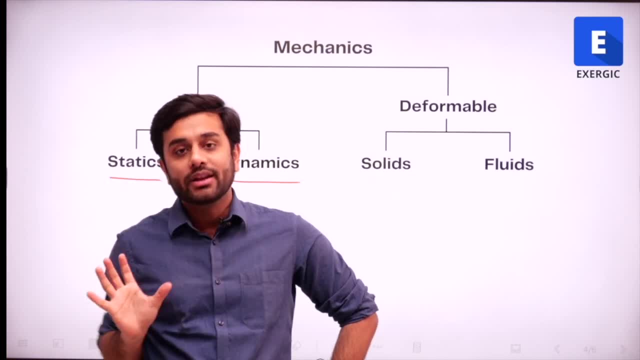 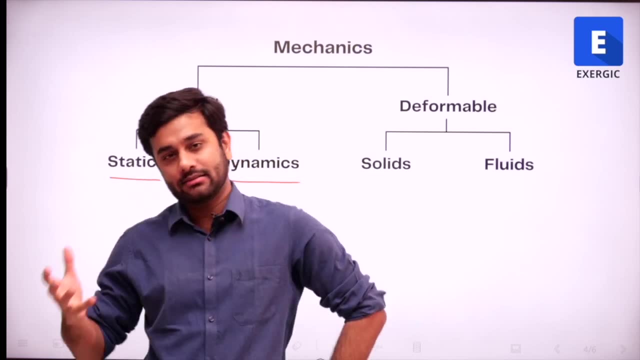 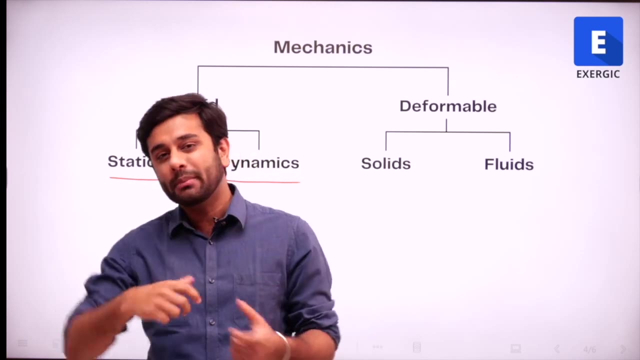 by considering the motion of the body, whether body is at rest or body has started to move. that is the criteria on which we discuss in engineering mechanics. right, in engineering mechanics. we have never considered the deformation, the twisting, bending, distortion of the body. right or not, that branch of study is. 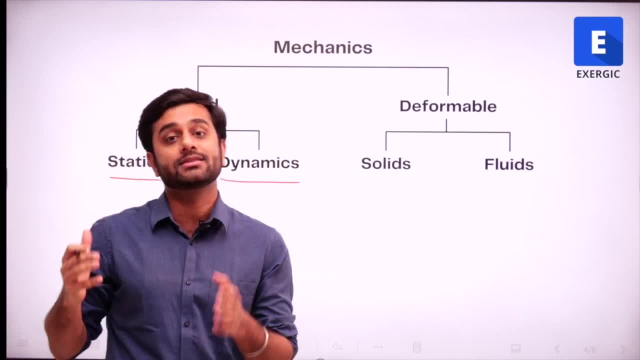 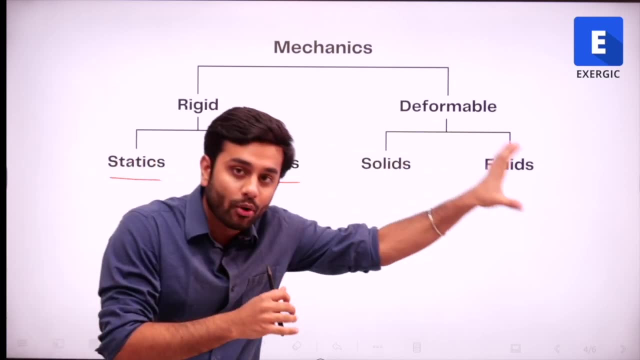 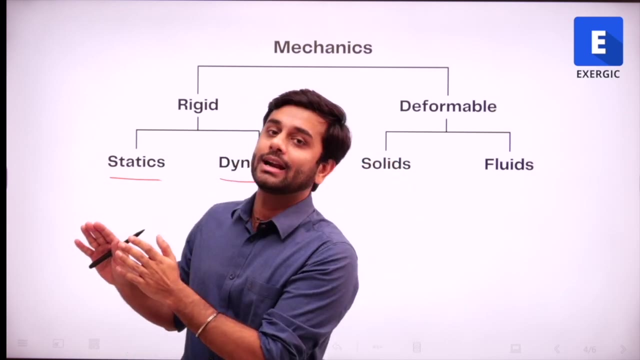 this one. it is called as rigid body mechanics. the engineering mechanics has another name, which is rigid body mechanics, where we don't consider the deformable bodies. even if the body is deformable, those deformations might be happening. but that is not the point of discussion at in engineering. 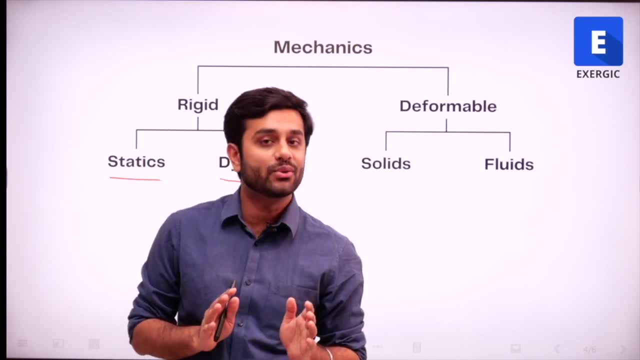 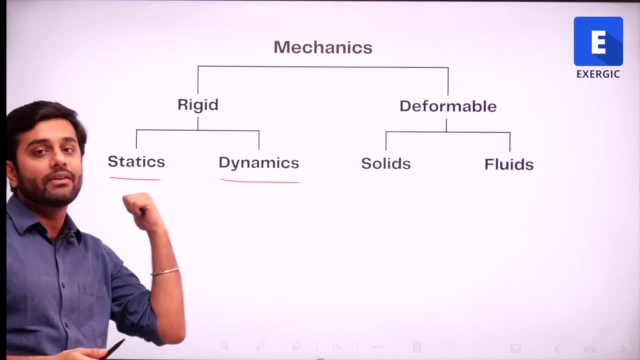 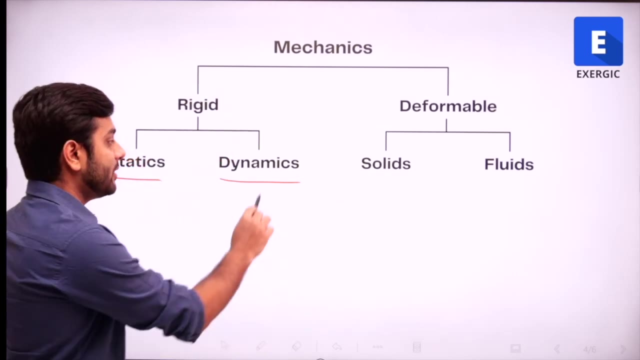 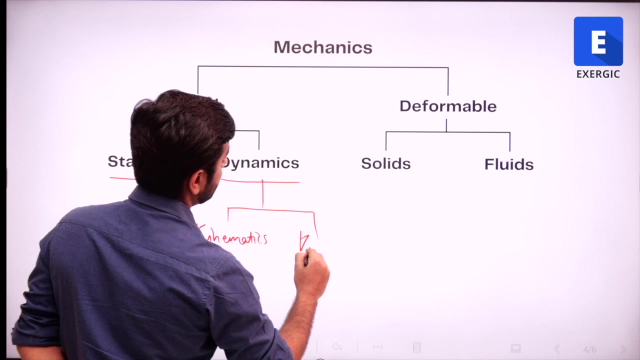 mechanics we are only concerned about the motion part of the force right. that branch of study is called as engineering mechanics or rigid body mechanics. this is further divided into other things, as i told you: statics and dynamics. this is something that we have already covered in engineering mechanics. then dynamics is further divided into kinematics, into kinematics and 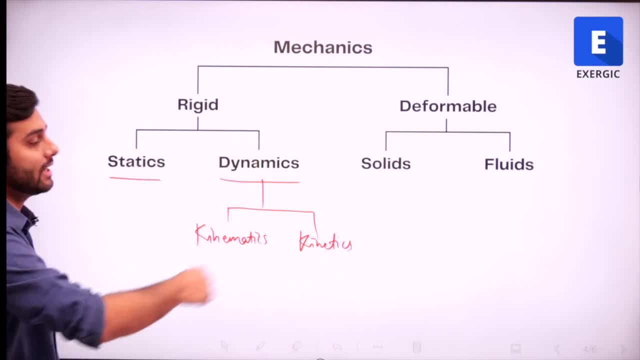 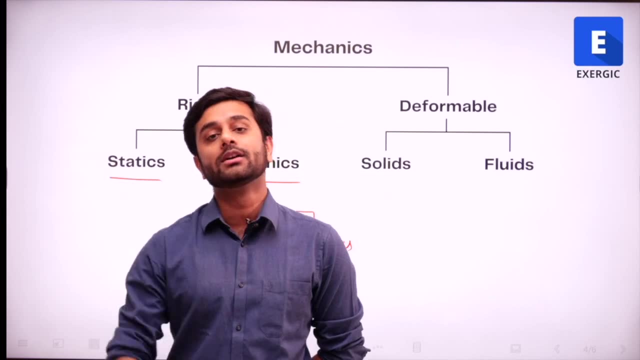 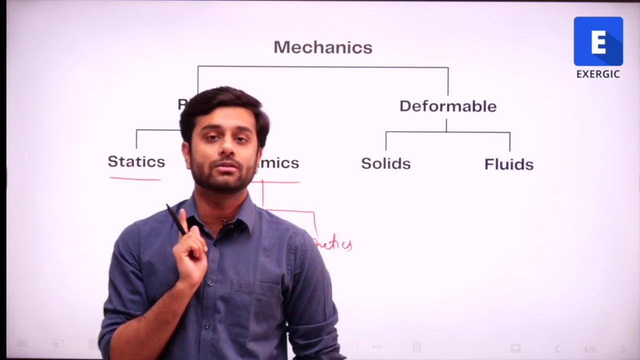 kinetics, right or not? this is something that we have already covered in engineering mechanics. at this point of time, i would also like to mention one more subject here, which is theory of machines. this is another design subject which we are going to cover. in theory of machines also, the parts are considered to be rigid. the deformation of the parts is not. 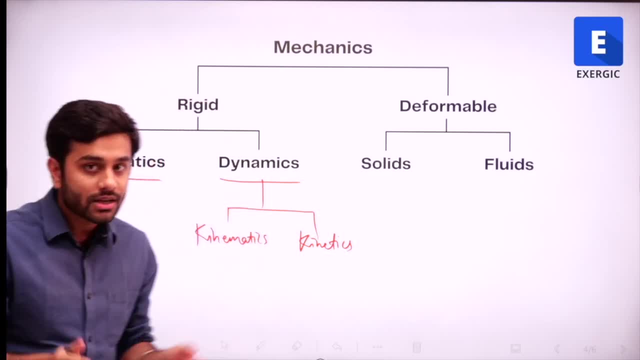 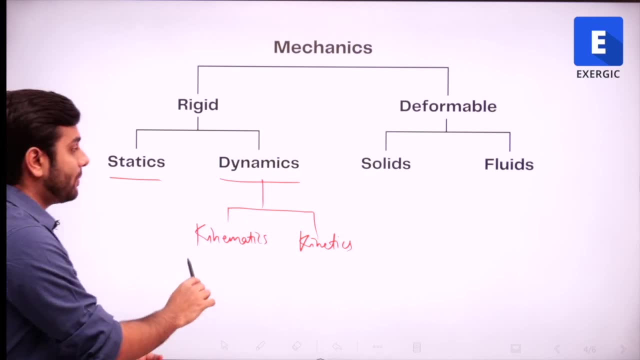 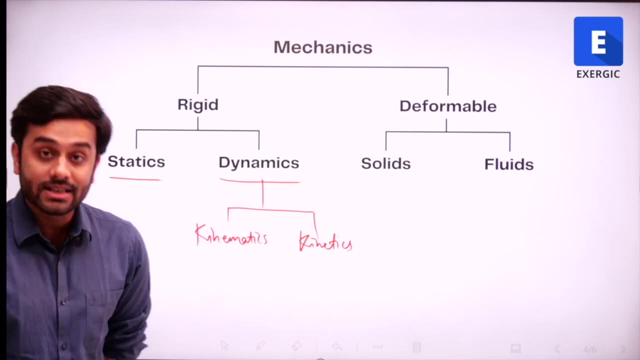 discussed. so theory of machines also comes under rigid body mechanics. you will find in some sources that you will be told that theory of machines is a part of rigid body dynamics. but that is not totally correct because in theory of machines also statics conditions also exist, when we will cover 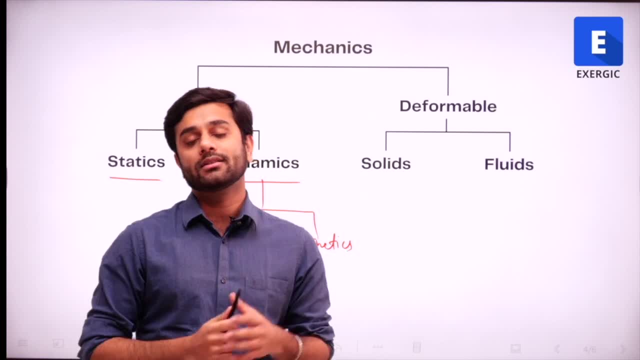 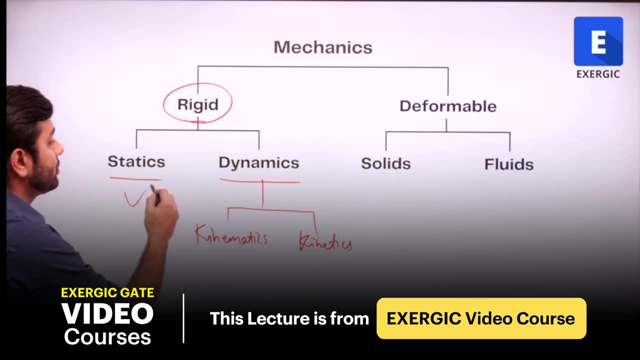 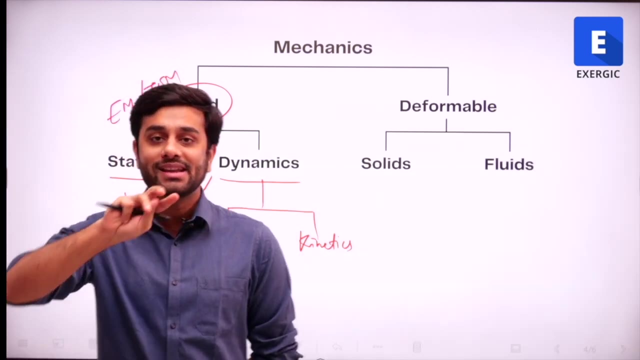 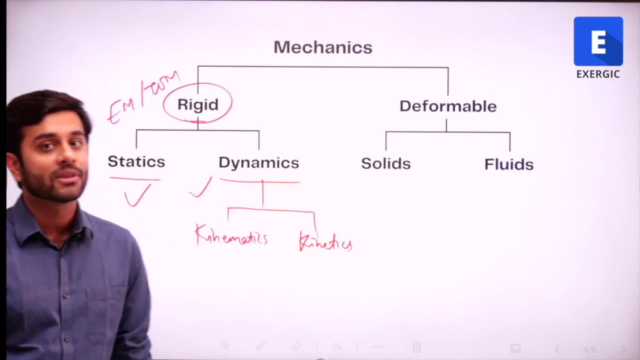 at gear trains and some other cases have static rigid body discussion. that is why theory of machines also comes under rigid body mechanics, where both statics and Dynamics are discussed. so, as you can see very clearly here that mechanics has been divided into different branches, which we deal as different subjects, so you can see how interconnected they are: mechanics and theory of. 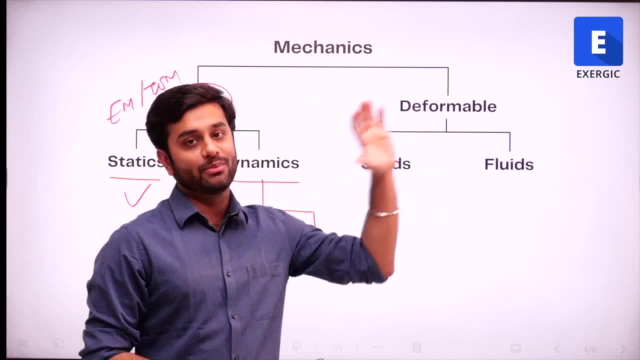 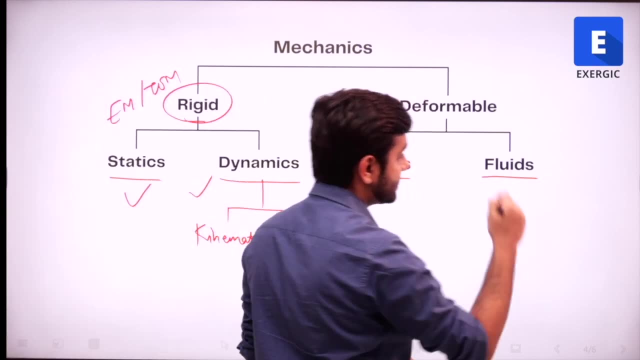 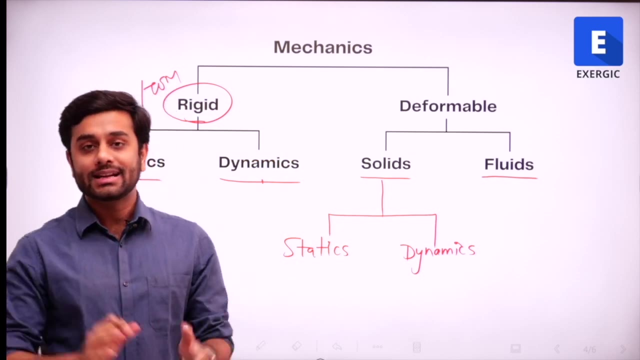 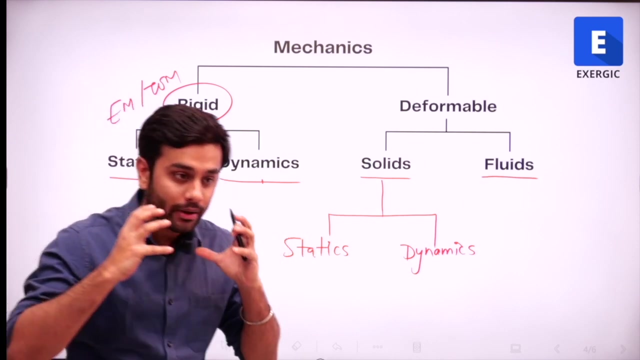 machines will be rigid body mechanics. and coming to the deformable part now, you can very clearly see two, two different classifications. one is solids, other is fluids. when we have a solid body which is deforming, you can further classify that into two different branches. one is statics, when the body is not in bulk motion, when the body is at its own place. 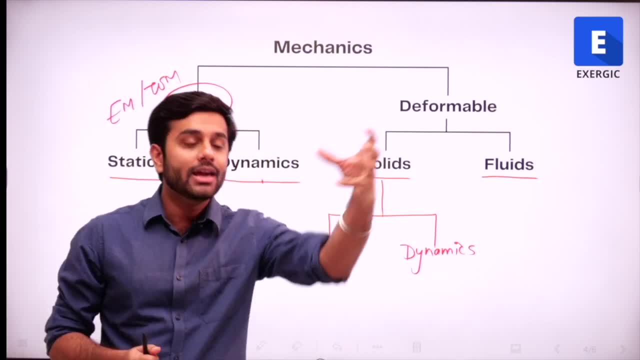 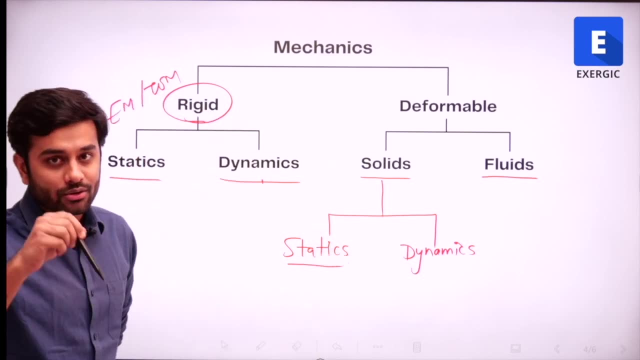 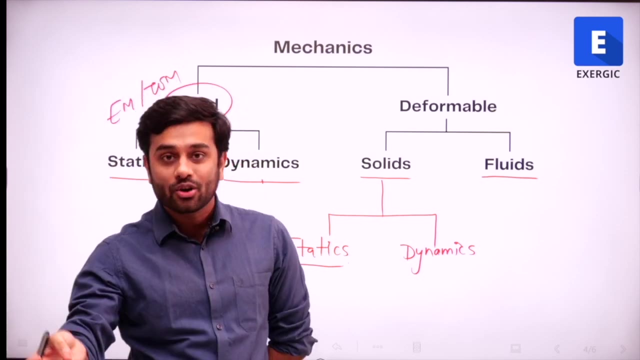 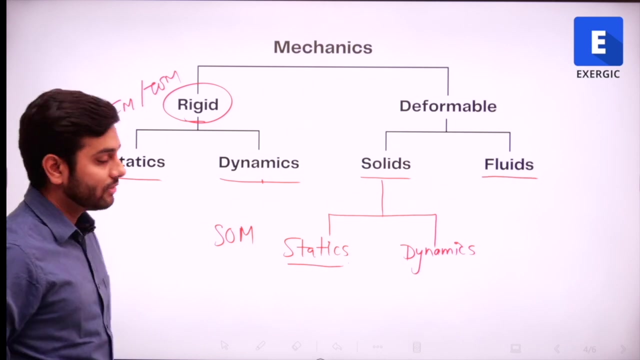 and the other is dynamics, when the body may dislocate, may start moving. this particular study comes under strength of materials. there are different names given to it: strength of materials, mechanics of materials, mechanics of solids- I'm sure you have heard of these names already. strength of materials, the course name that we are having right now. 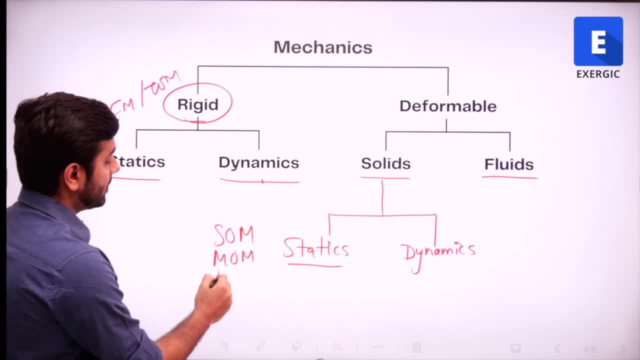 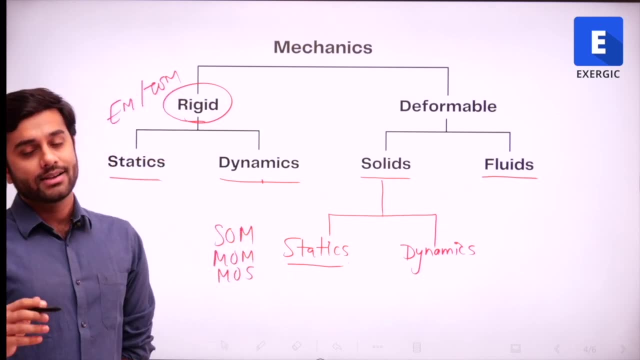 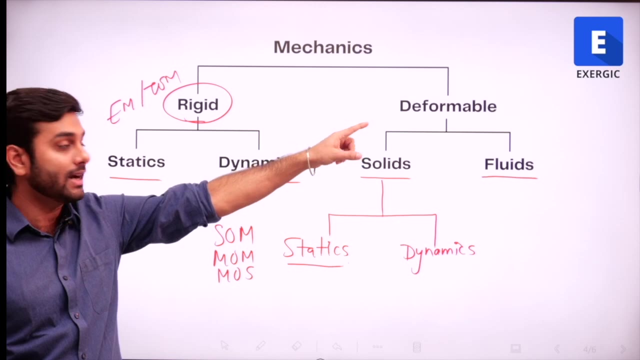 mechanics of materials, MOM, mechanics of solid mos. these are different names for the same subject. as see, it's a type of mechanics only, but a deformable mechanics which in which we will be studying about solids under statics. So this is the exact position of 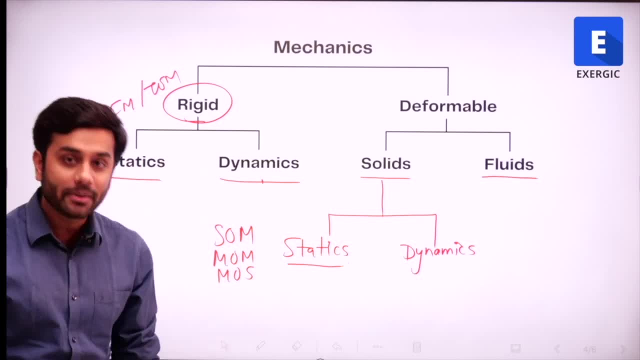 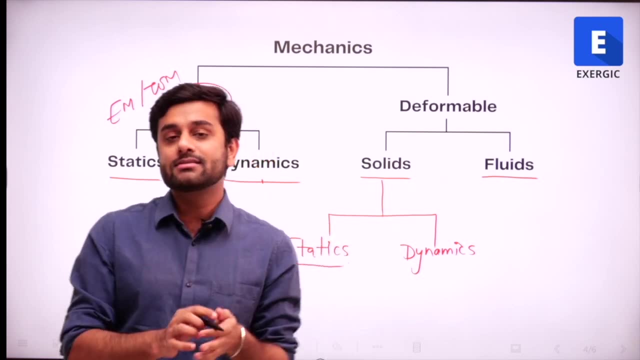 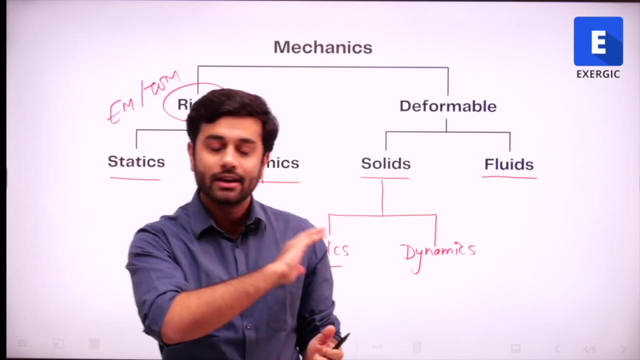 strength of materials in this whole tree. At the same time the dynamics, part of solids, deformable solids, we study in vibrations. Vibrations is in our course, is a part of theory of machines only as such. it is mentioned in Gates-Celebers separately- again a very important discussion- but in our course it is. 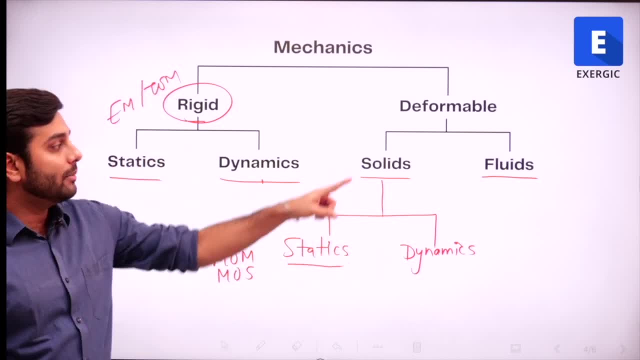 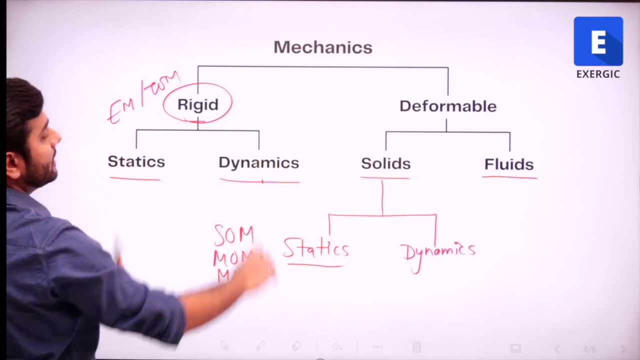 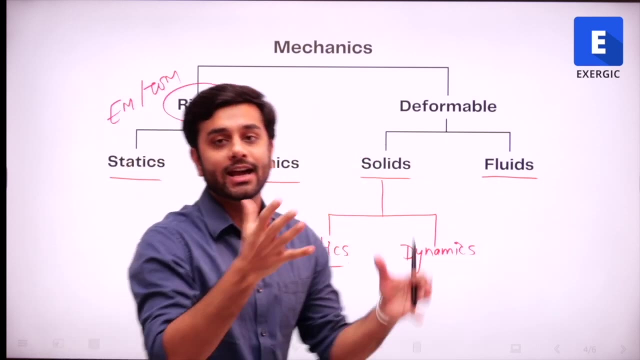 taught within the theory of machines itself. Coming to fluids, fluids again are divided as the same: statics and dynamics. as you can see, this is also divided in statics dynamics. this will be also divided in statics dynamics. Fluids again are divided into statics and dynamics. Dynamics again will be divided. 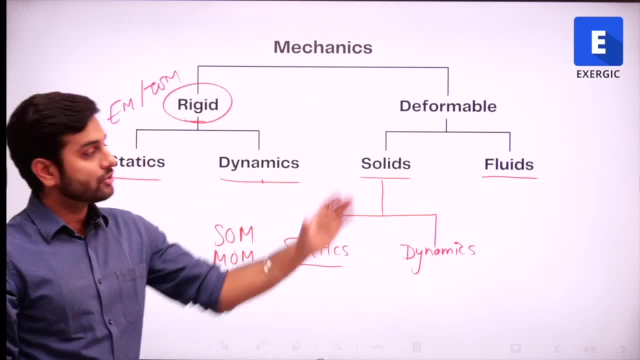 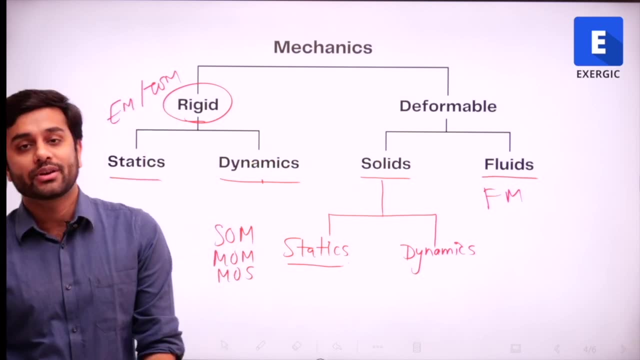 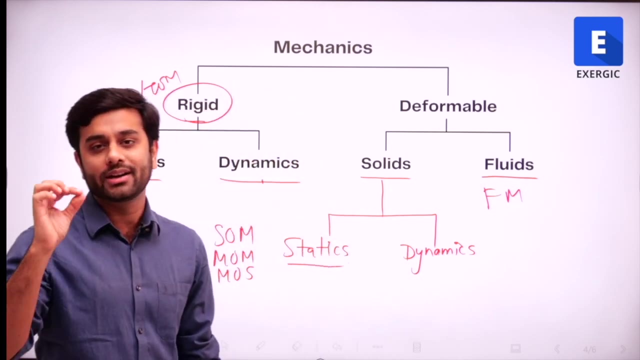 as I told you here, kinematics and kinetics, So that complete discussion of fluid is again a subject which we call as fluid mechanics. So, as you can see that from a single branch of mechanics, how many different subjects are coming out, If I exactly point it. 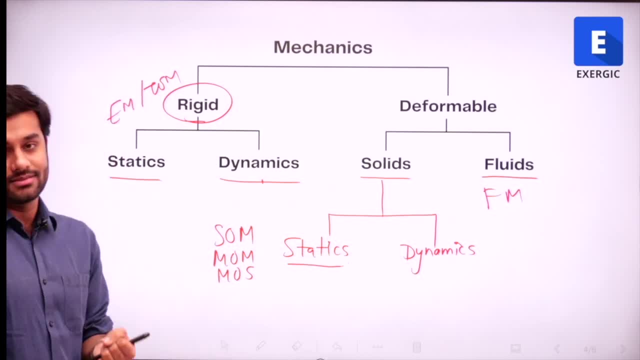 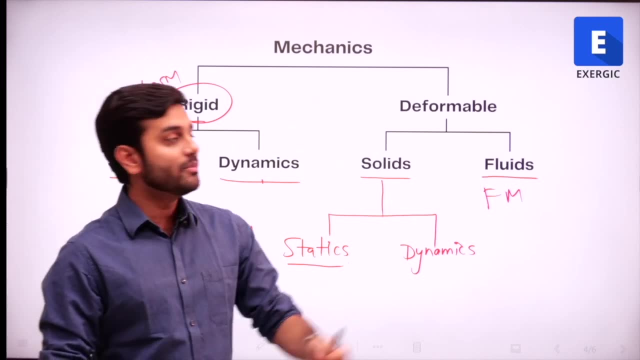 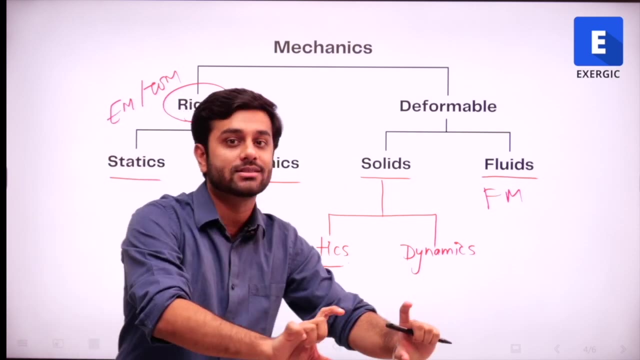 out from the Gates-Celebers, then mechanics is a subject, theory of machines is a subject, strength of materials is a subject that we are going to discuss and we have started it. Fluid mechanics is a subject and the vibrations that we are going to study. that also in the Gates-Celebers is a separate subject, although I will teach that.